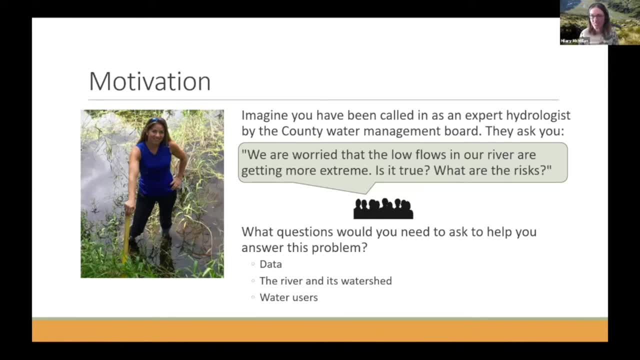 we're worried that low flows in our river are getting more extreme. Is it true? What are the risks? And I asked them to think about what kind of data and information they need to answer this question. So this is the kind of question that we'd like the students to be able to answer. 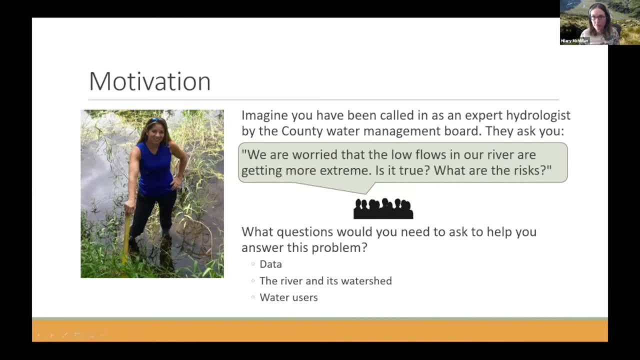 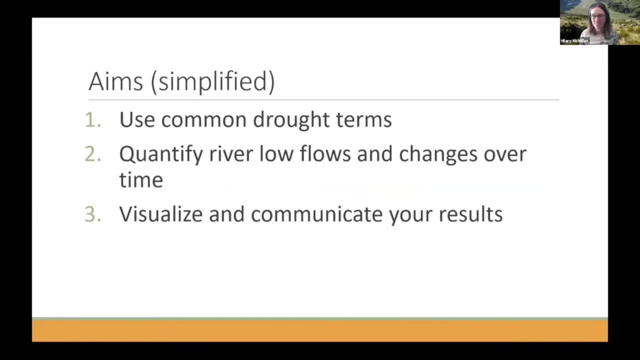 after they finish our module. So, in terms of the aims of the module, in very simplified terms, we want the students to be able to do three things. They finish the module So to be able to use common drought terms and know what they mean. 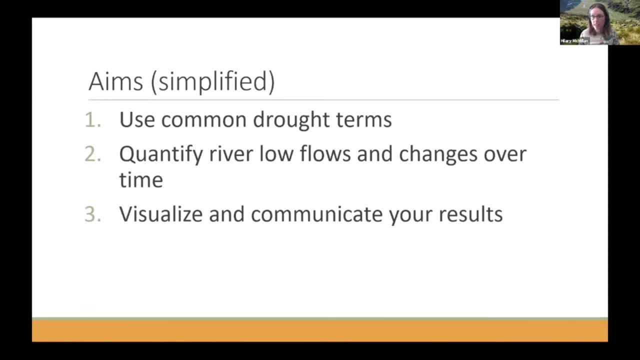 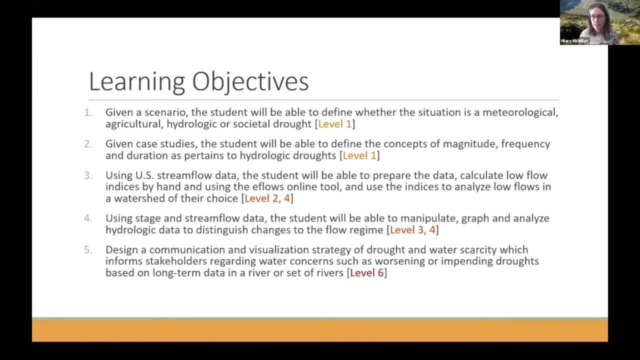 to be able to quantify low flows in a river and quantify how they change over time, and to be able to visualize and communicate their results. So we turn these simple aims into the learning objectives that we have for the module. So they're kind of divided. 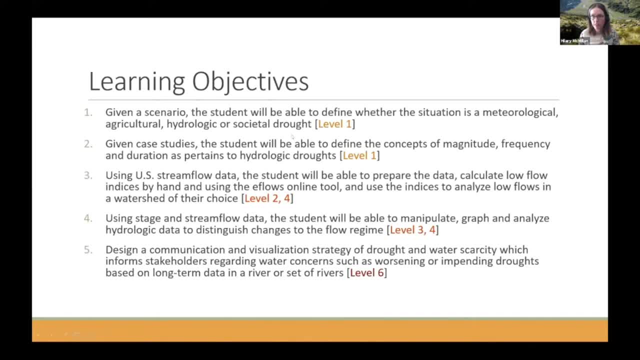 into three parts, So the first two are more simple ones, about the defining a common drought term. So we want the students to be able to say whether a situation is a meteorological drought, agricultural, hydrological, societal drought, And we want them to be able to define the concept. 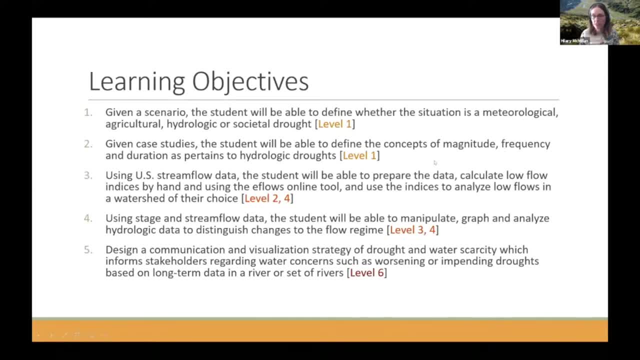 of magnitude, frequency and duration as we use them to define droughts. We then have two higher level objectives, which are more about processing the data to be able to understand how low flows change over time, And we then have a final objective which is at a higher level. 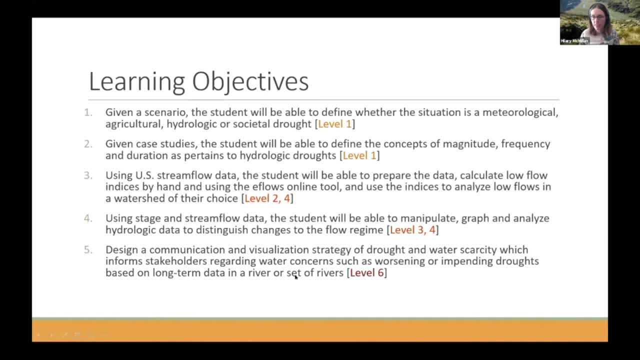 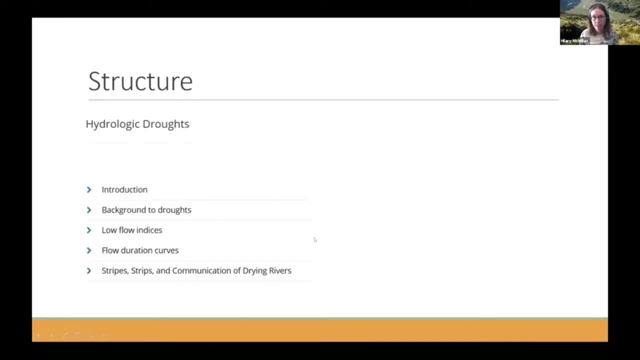 where the students present the work that they've done and use different visualization techniques to describe how droughts have been changing. So in terms of the structure of our module, then this is how it looks like. So it's basically got a background section. It's then got two sections on low flow indices and 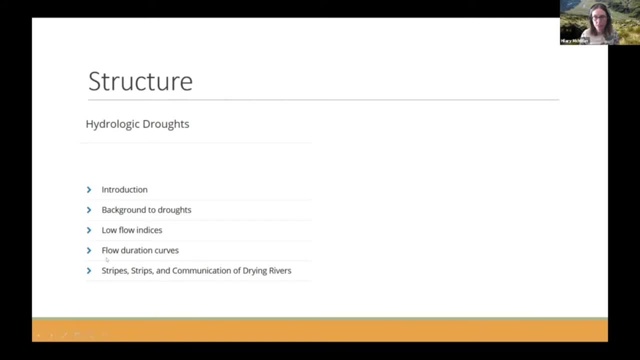 flow duration curves where the students are working with data and processing it, And then it's got a final section on visualizing and communicating their work. So, unlike, I guess, the other modules that we saw earlier then we don't use one specific case study. 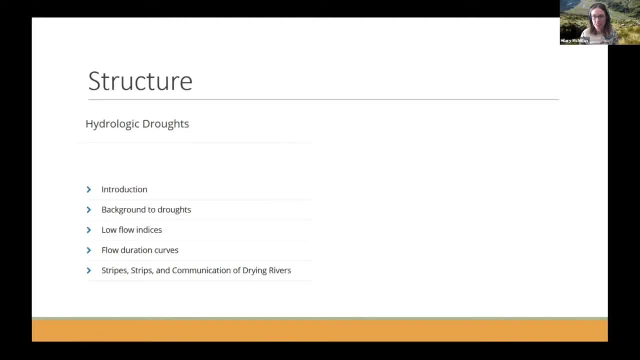 But throughout the module we're inviting students to use their own river that they're interested in and download their own data and then work with that data. So then, hopefully, if you do this in a class, then you end up with a nice variety of different watersheds that the students have worked with. 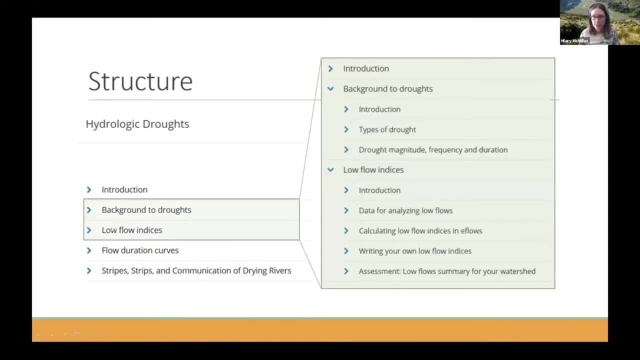 So I'm going to talk about the first two sections briefly and then Joanne will introduce the second two sections, So just to give you an overview here. So this is their background section, learning about the drought terms. And then this is the first of the two quantitative sections. 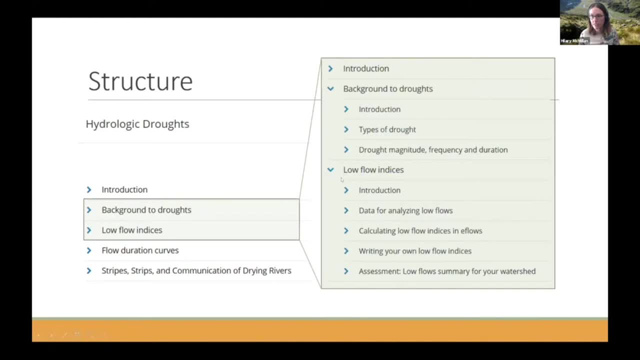 where they're going to calculate various low flow indices for the river. So index, a low flow index is things like what's the number of days per year where the river was at a zero flow, something like that. So like a quantitative way of saying how low the river flows are. 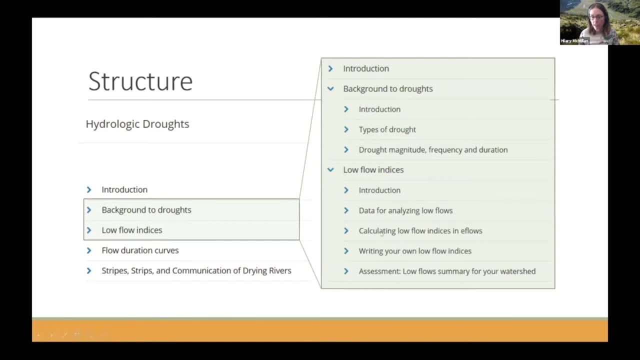 So they're going to do that in two ways. They're going to use the eFlows tool, which is actually something that Belize has been involved in developing, but it's a really nice web tool where they can upload data from their watershed and then 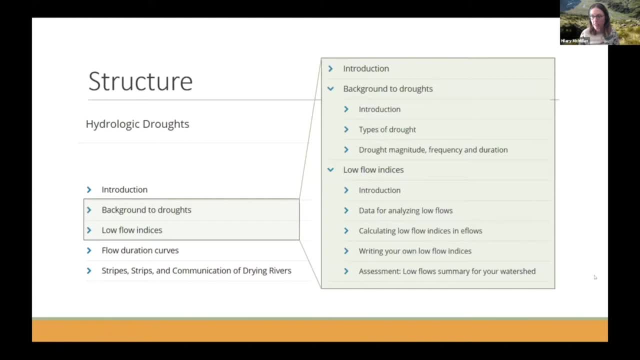 automatically calculate various indices. And then the second part is that they're going to write some of their own indices. So this helps them to actually see what's going on behind the scenes of a tool like eFlows and actually process some of their own data. just 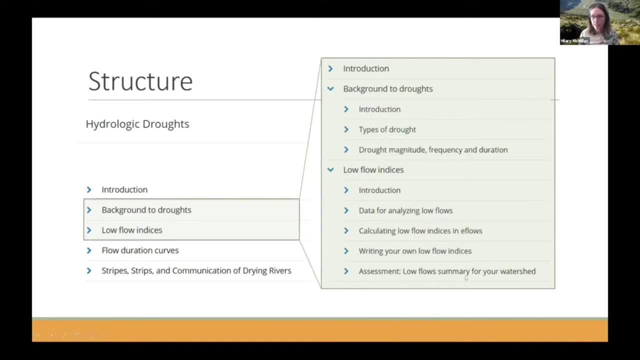 using a spreadsheet, And then they have an assessment to write that up. And then the second part that Joanne will talk to you about is about using flow duration curves which visualize the cumulative distribution function of river flows and how they change. And then 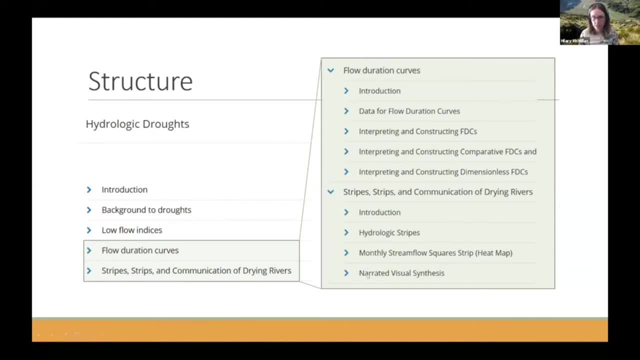 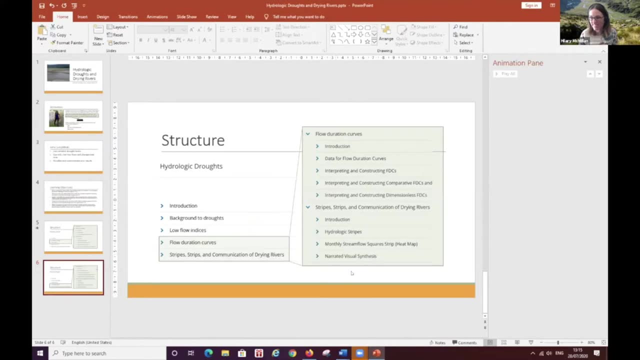 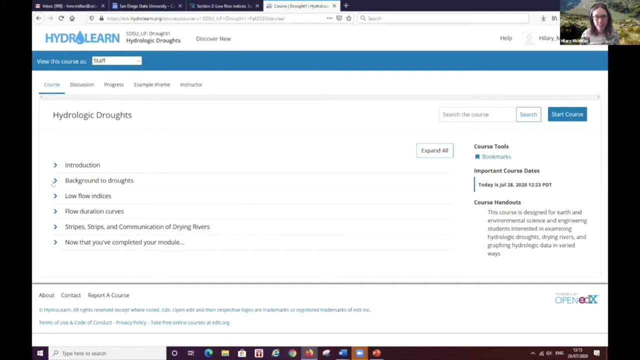 the part about visualizing and communicating their results. So I'll just switch over to. I can't work this technology. I'll switch over to the module. Okay, so hopefully you can see this module now. So here's our module And this is the. 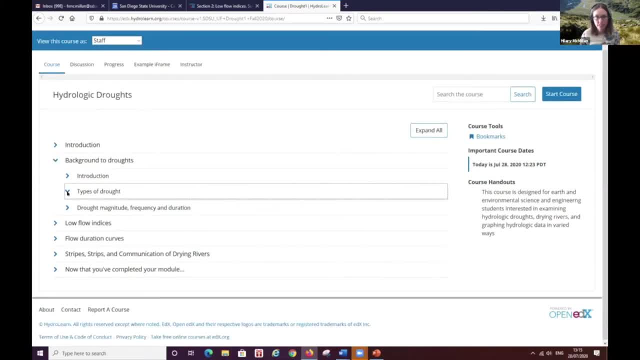 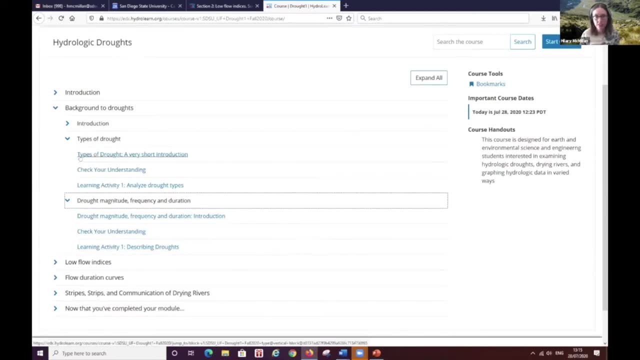 background section And so the background section. if I expand those, you can see that these have the same kind of outline So that it introduces the student to the topic. There's a short check, your understanding quiz and then a learning activity which basically asks: 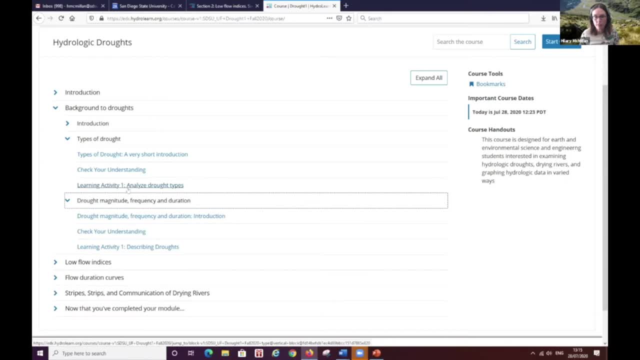 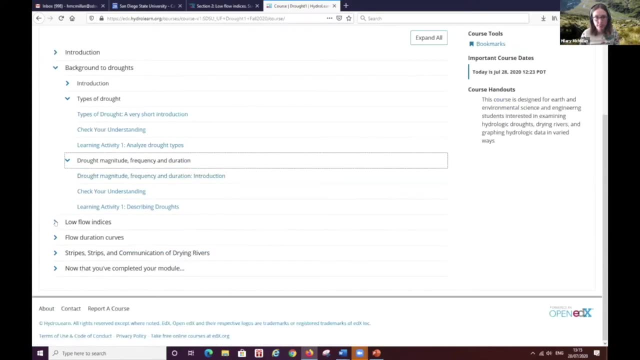 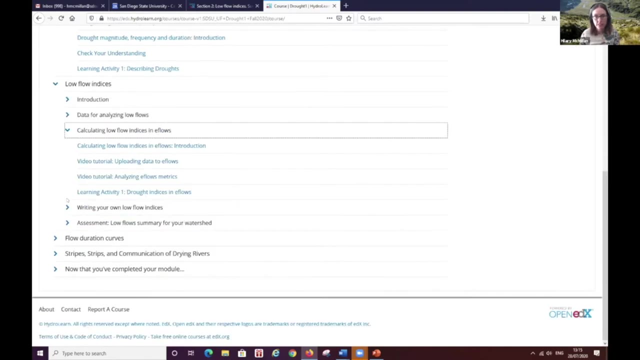 you what's going on behind the scenes. And then the second part is that they're going to to do a reading and then produce either a discussion post or a short discussion with their partner. And then here's the section on low flow indices, And if I expand these, you can see. 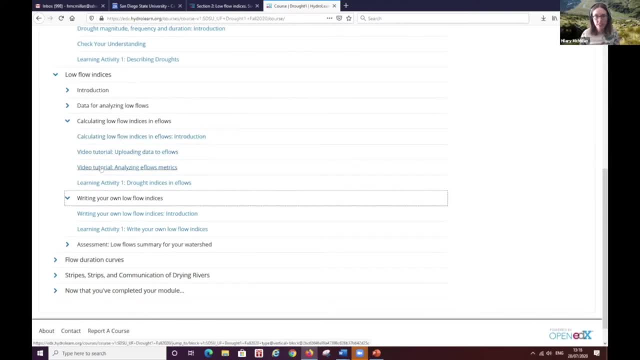 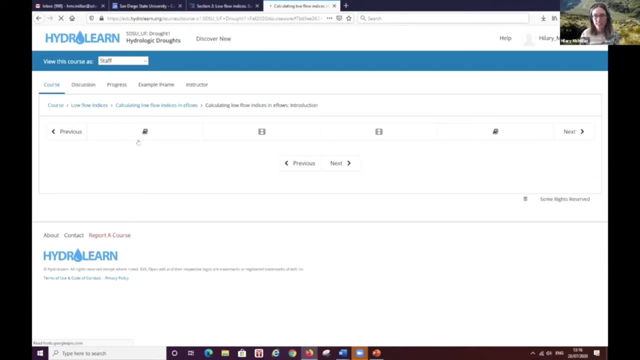 that they each one has an introduction and then some tutorials and then a learning activity, And I'll just show you this first one as an example. So here's the first one, And then the second part is their introduction to the low flow indices using the eFlows tool. So it gives them a lot of. 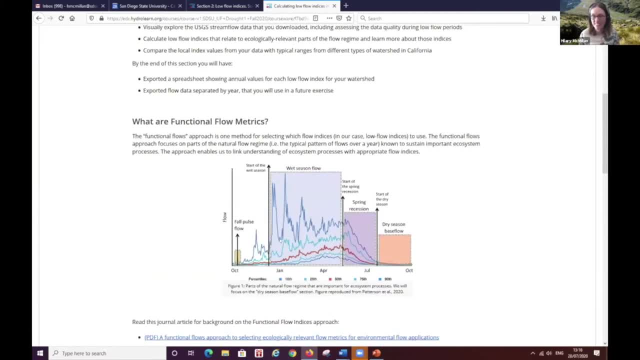 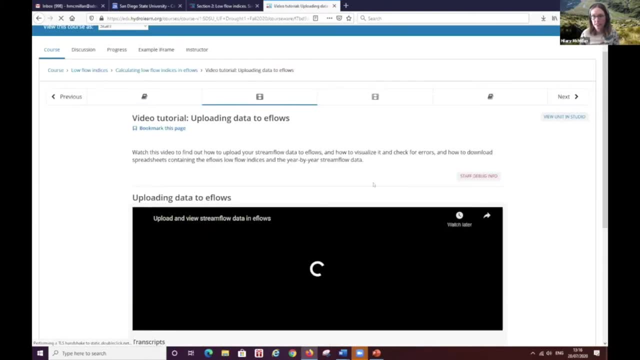 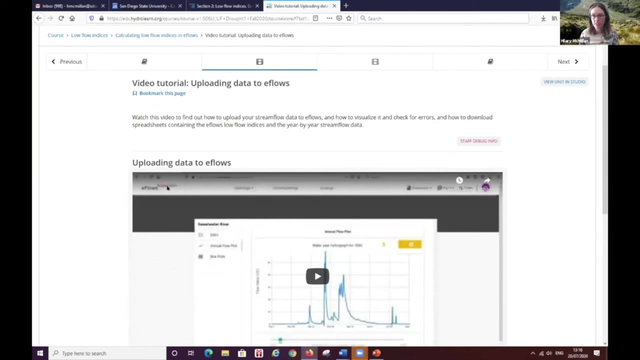 background data steals one of the pictures from the website to explain what they're going to achieve. And then, if we go next, then throughout the module we used various different ways of of explaining the methods to the students, But in this case, then, I've created some video. 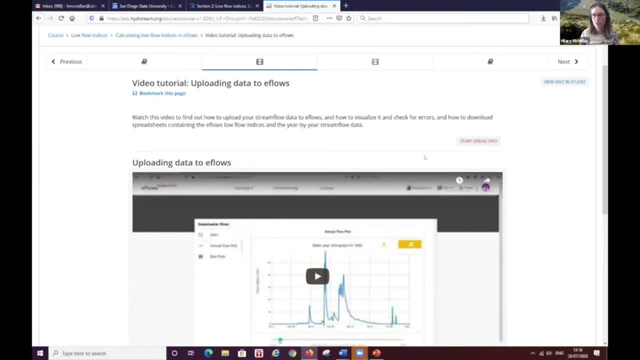 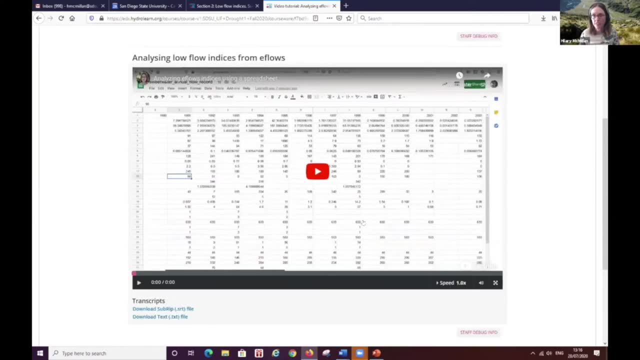 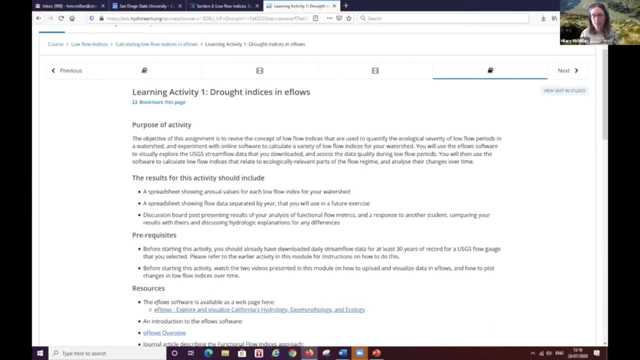 tutorials so they can follow along while I go through the activities, and then they can see what they're doing And it shows them how to process the data into the spreadsheet. And then at the end there's a learning activity which asks them to having been through these activities and 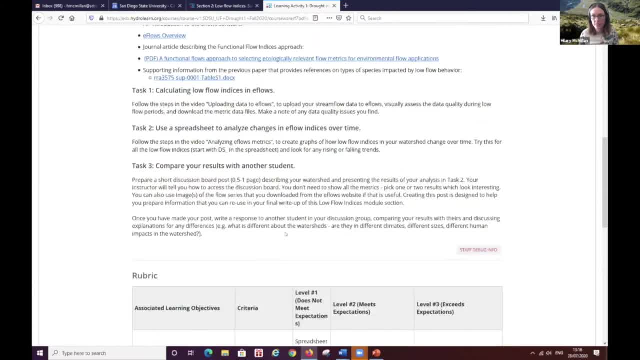 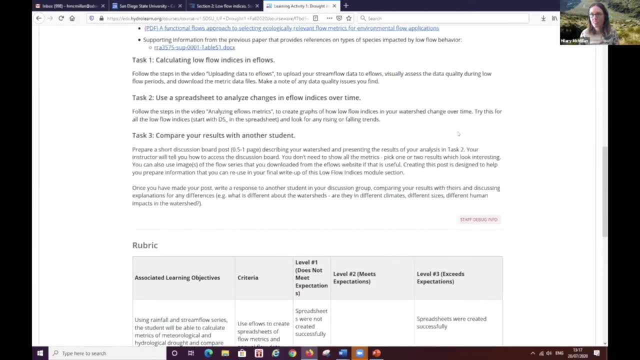 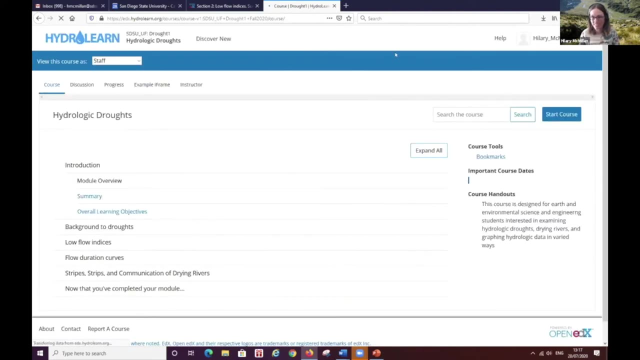 they can write up their results, shows them some supporting data, asks them to compare their results with a with another student, And I think I will go back to the course. I can't see the chat, but I think I got a five minute warning, So I will pass over to Joanne to introduce the second two parts of the module. 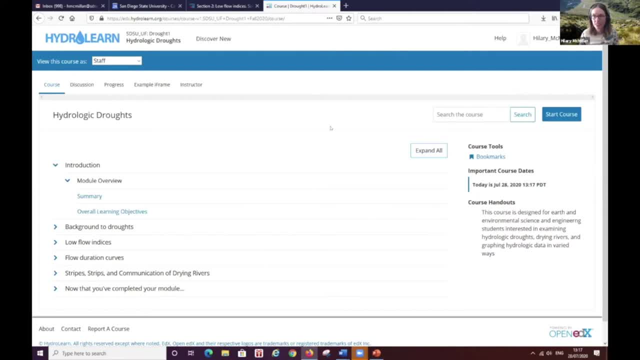 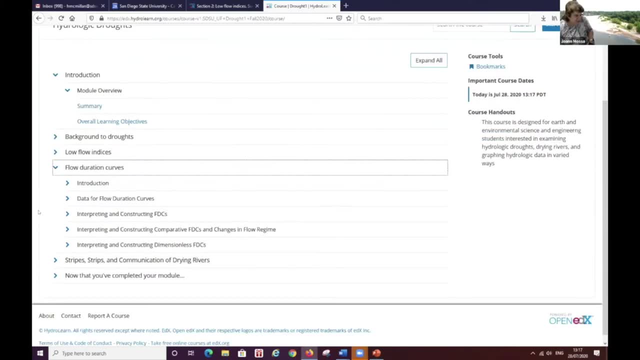 Okay, Joanne, do you want me to drive the screen or do you want to take over? Yeah, you can drive if you want. Okay, So the flow duration curves module is structured similar but a little bit different to Hilary's in that what I've done with the check, your understanding is put them in the first two. 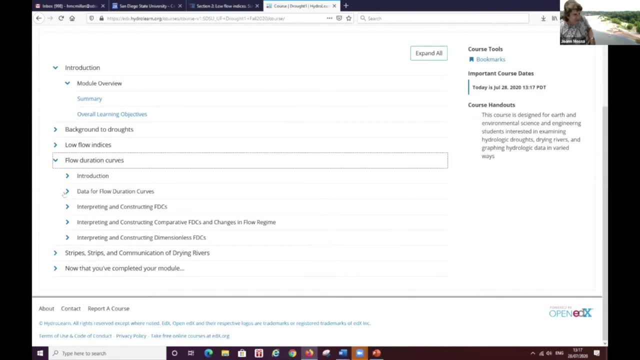 first few sections Where they're learning about things, and then later on then the you know they actually do the activity. So you know, one thing I was finding was there were so many different pages for students to go to that I wanted to sort of combine them into one page. 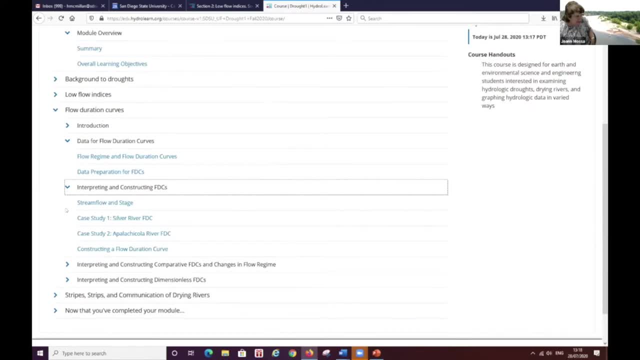 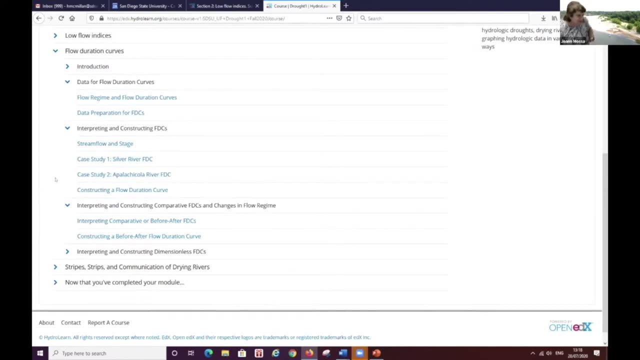 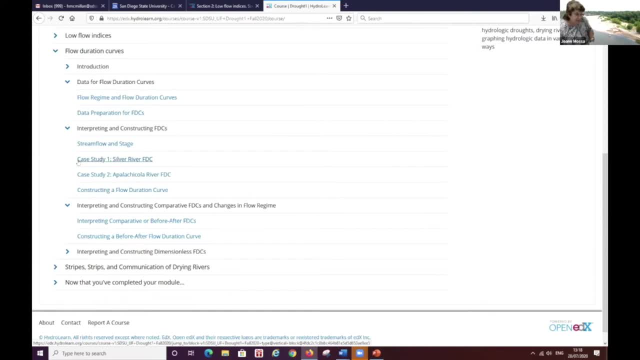 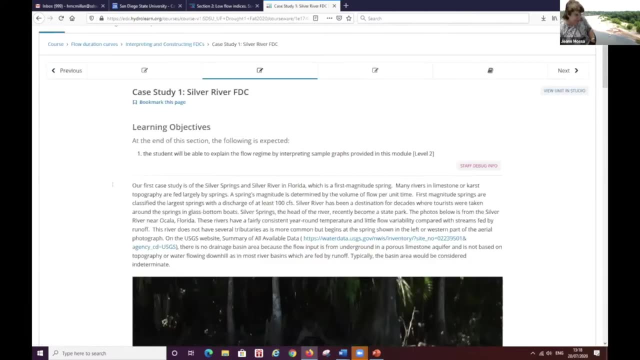 Okay, So one you know again, you can do multiple choice and find things. One of the great home messages for students is you can have rivers in a very humid climate, like Florida, And these rivers can be drying due to, in this case, human activities. 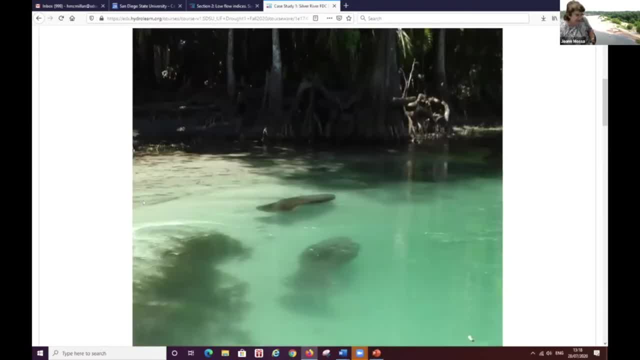 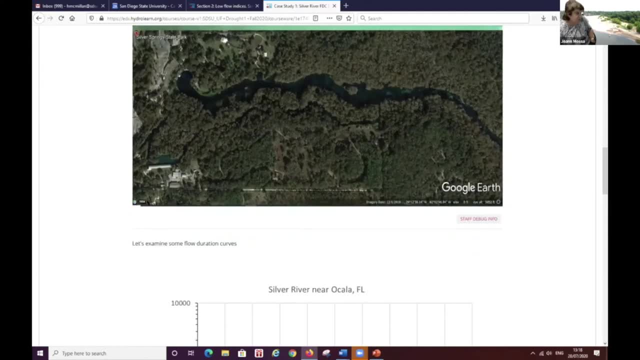 And so the silver river is a spring fed river, And Hilary is going down and showing kind of some of this story in graphics. So it actually doesn't have any measurable drainage area because it's fed by groundwater, And so we have some sea level control. This is the slow-mo that we have today And, as I mentioned, there are two parts of the data. So one is this: this is the high water flow. So the other part, we have these little circles of these little circles of the water. 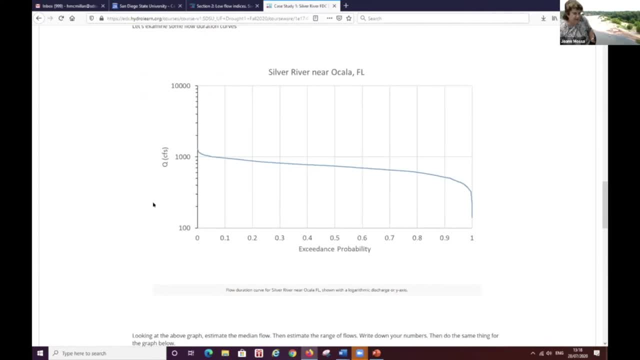 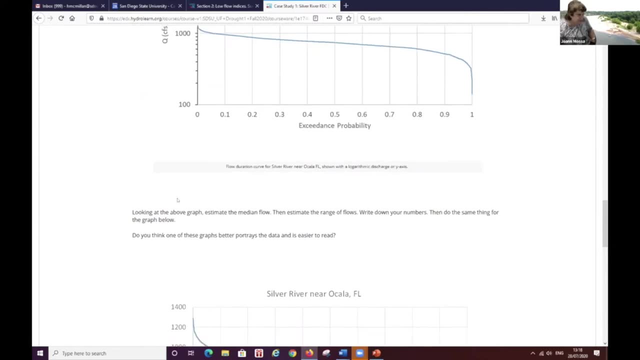 And this difficult layer here. The bottom one is the surface groundwater, And so we have some sample flow duration curves of this, And then the other river, which is the Apalachicola River, which has a large watershed. We talk about the difference. 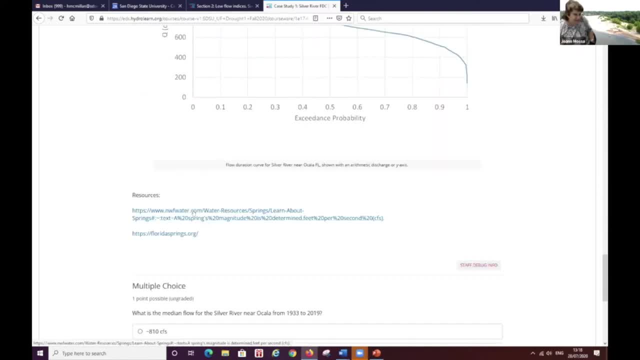 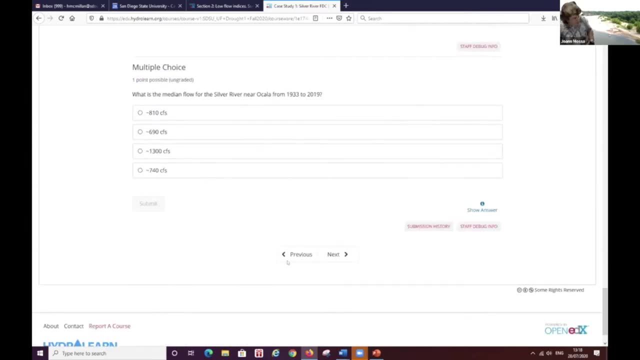 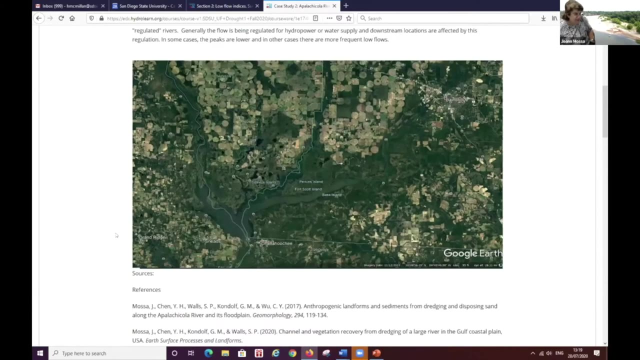 between plotting on a arithmetic and a logarithmic axis and a little bit about how to interpret this. with a check your understandings at the bottom, You can go do the Apalachicola next, I guess. And so here we have a reservoir and central pivot irrigation And we have some nice graphics. 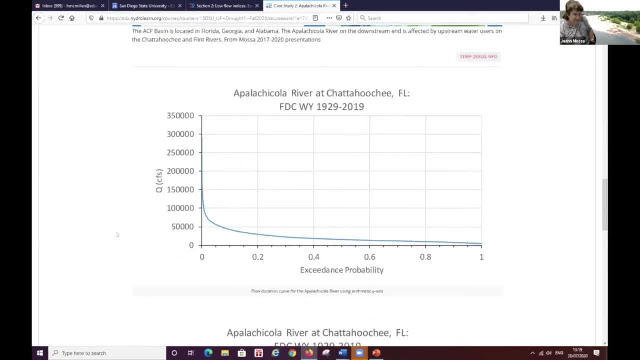 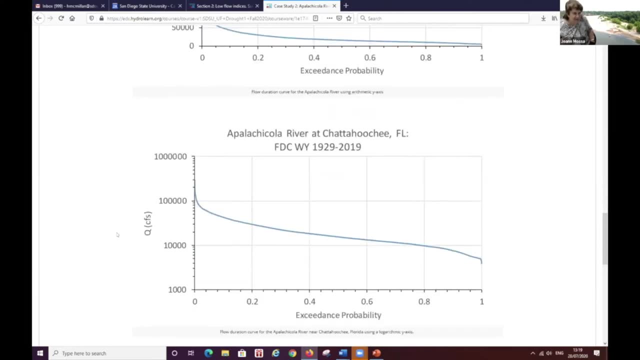 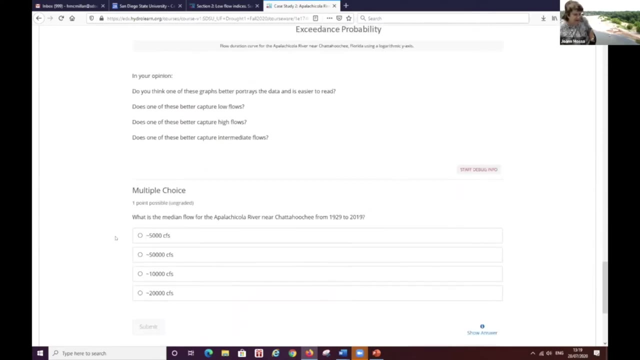 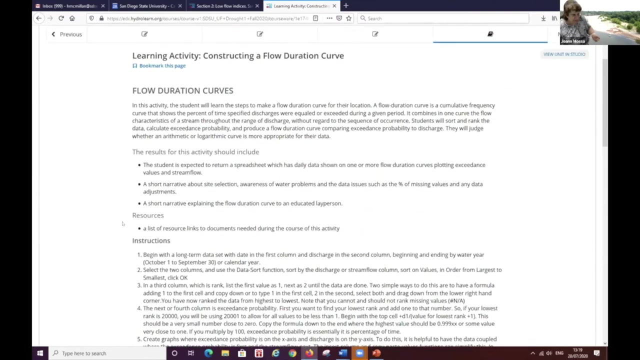 that just show people that this is a different area. We have the flow duration curves. We get students thinking about which type of graph shows the data the best, And then some questions at the bottom. So we have a flow duration curve, a dimensionless flow duration curve and a 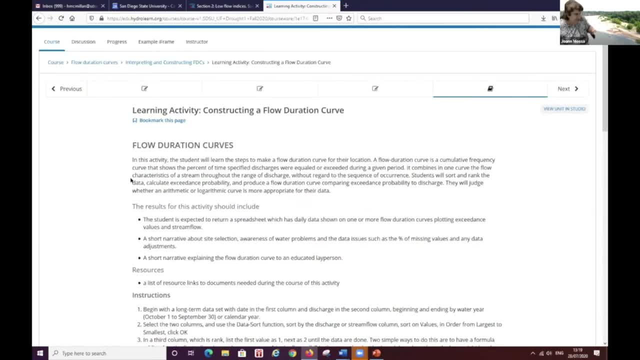 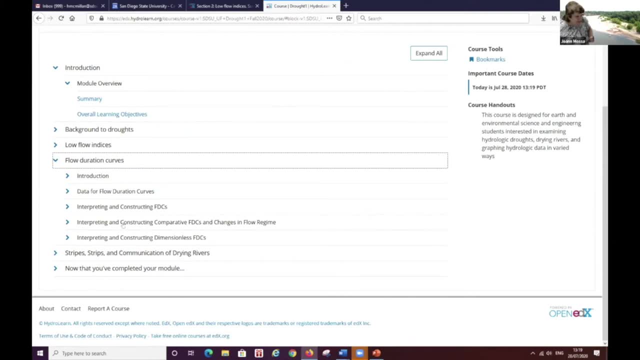 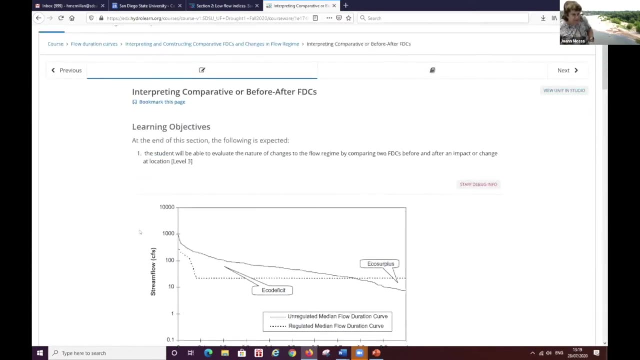 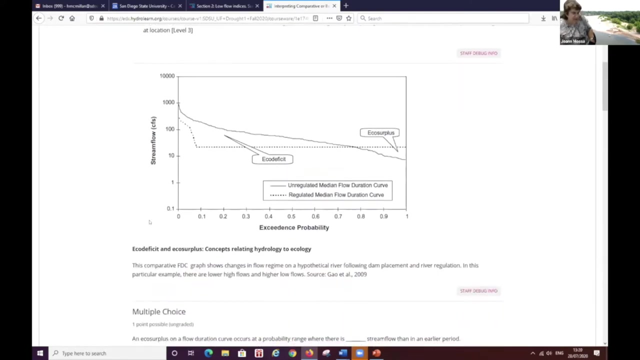 comparative flow duration curve And let's go to maybe a comparative flow duration curve, Just interpret, I guess, And yeah, just interpreting, constructing, and then we'll go to constructing too. So you know, in this comparative, I want to present the idea that once the flow regime 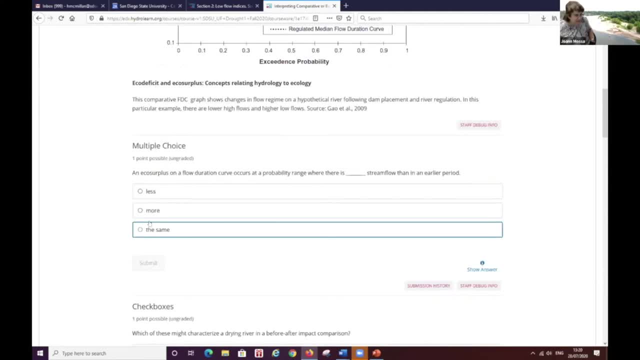 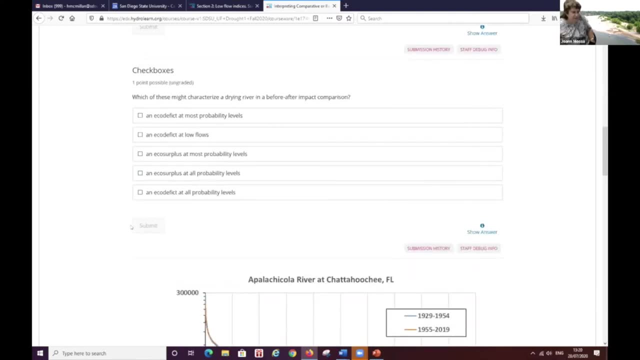 changes the Rate, weights are going to change too. So here's the constant cube and it changes too, the Lعت to the S one And the L形 it's going to also be changing too. Yeah, those things are. those equation types are going to vary, So of course you can interrupt gu Testament. 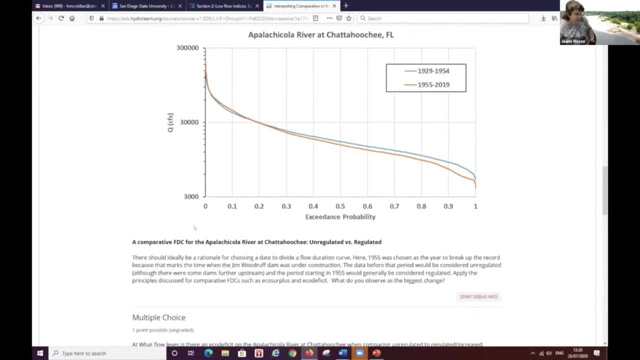 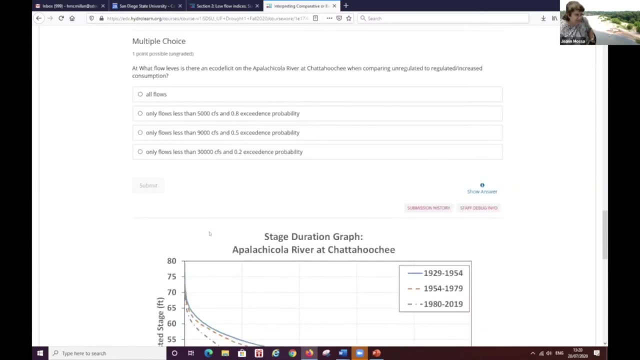 map with some macrolike statements. And also, if things happen, you can interrupt gu system mapping and we- or the system would have to- are working on that same thing too. And I like to think about the pointed三 bones. you can see the ten and five people. 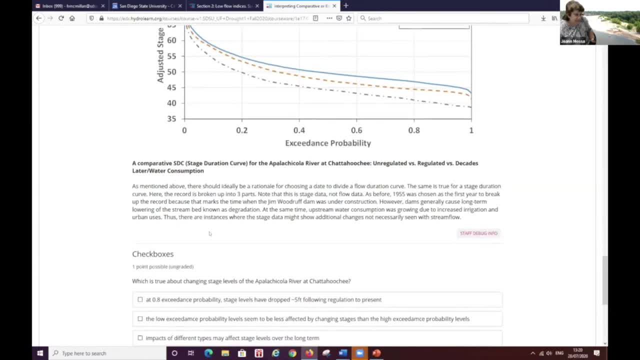 We're in the middle of a Y axis. Let's think about the was sort of a lot about how, what we're to that you can also have a big difference if you're looking at stage, and here I've actually looked at three time periods in this graph, And so they. 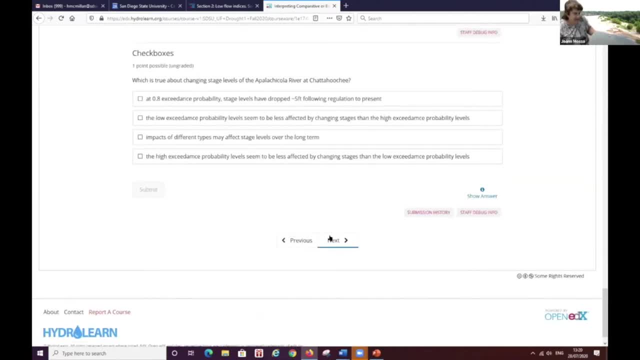 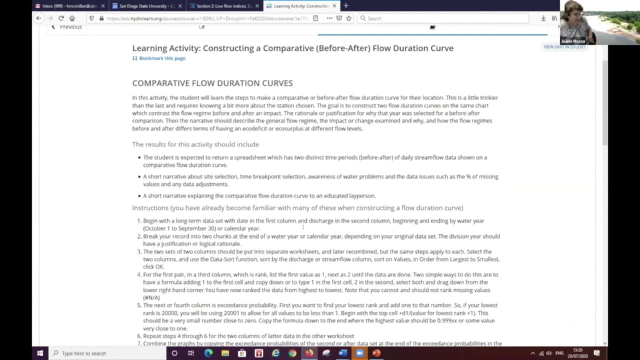 get the idea of how this can be applied, this method, and why you would want to pick certain breakpoints and how you can go ahead and do that. And so in the learning activity over here, you know I've listed the steps and then 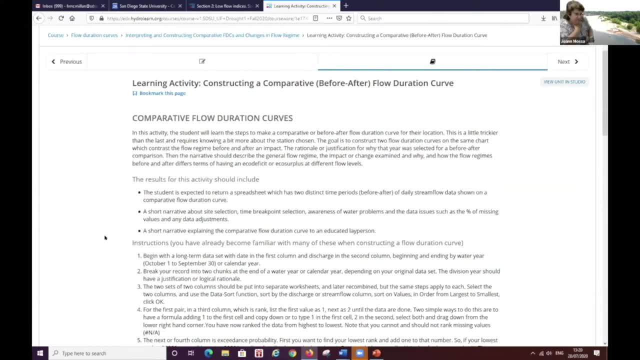 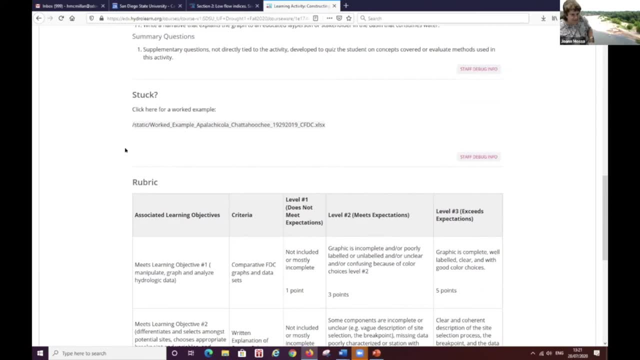 at the bottom. go to the very bottom. yeah, we have. I have a section called stuck and there's a an Excel spreadsheet that students can look at an example, And this is in all of the the modules over here, just so students can see. okay, your. 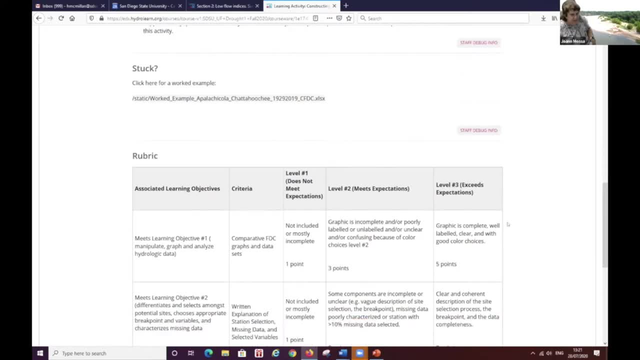 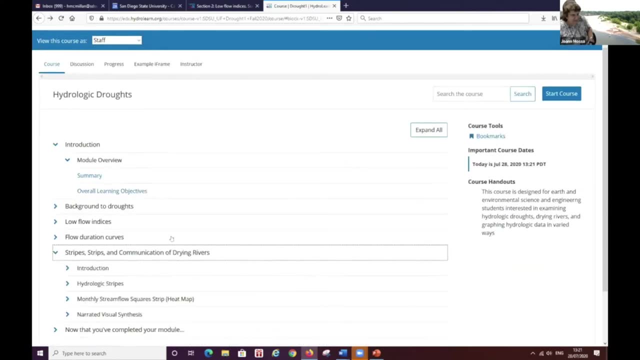 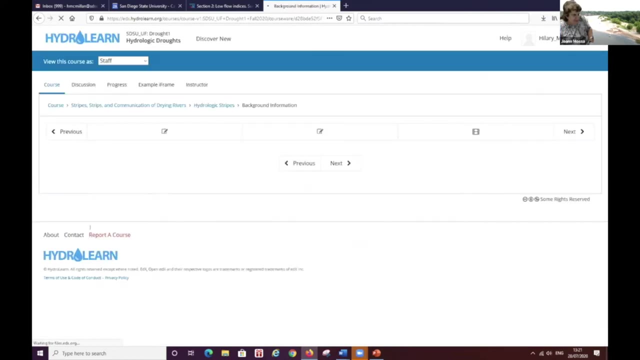 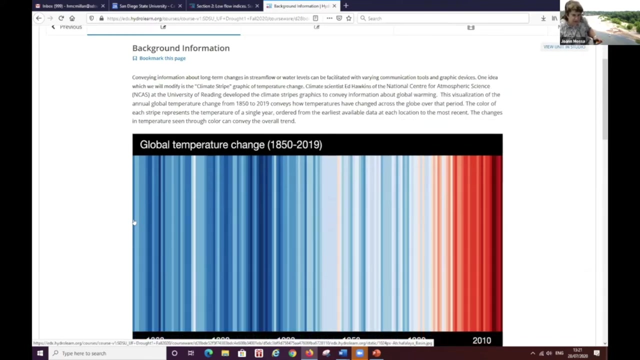 data are supposed to look like this. So, anyway, let's go to the stripes, and strips, I guess, next, and so this is start with stripes, I guess, And so the idea behind this, as this is an idea that was adapted from the climate stripes, which is a communication. 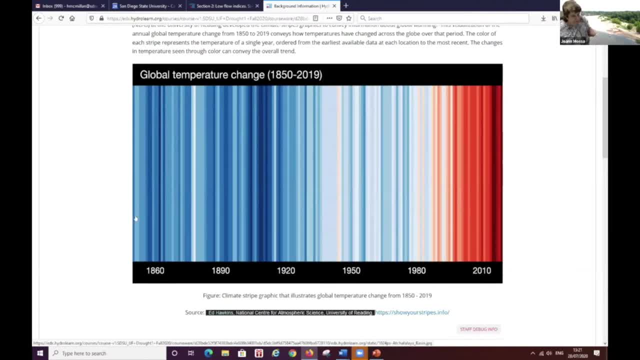 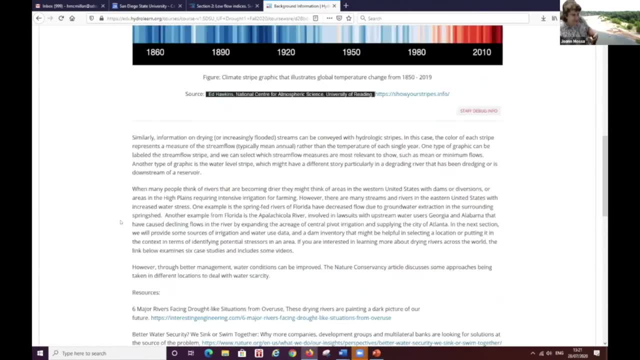 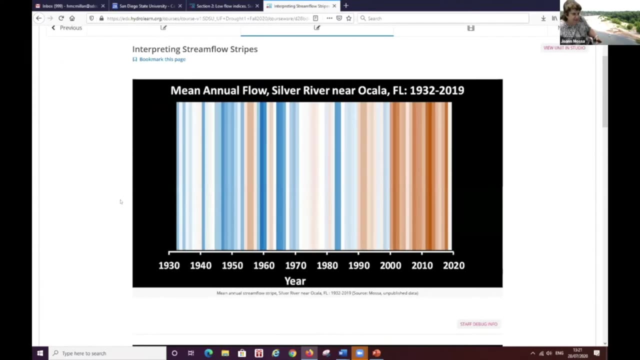 mechanism of trying to show that the world is warming through colors, And so you can see the blues changing to reds, and so I'm applying this same method to streamflow. So we go next, And so here I have two case studies of these two rivers that they've 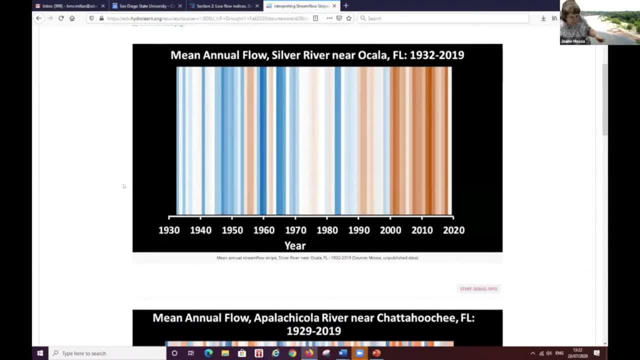 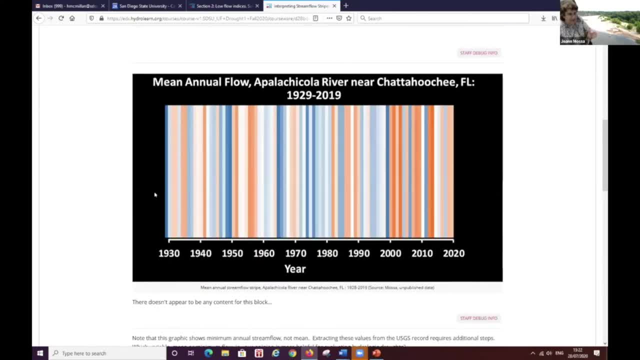 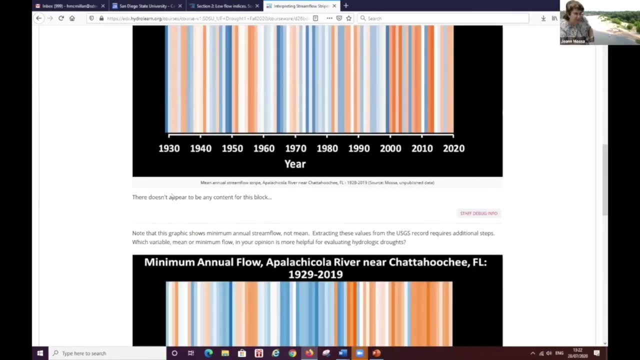 seen before: the Silver River in Florida and the, the Apalachicola River, and this is both with mean annual flow. but there's also an example below that with a minimum annual flow, if students want to extract further, and then you can really see the drying and 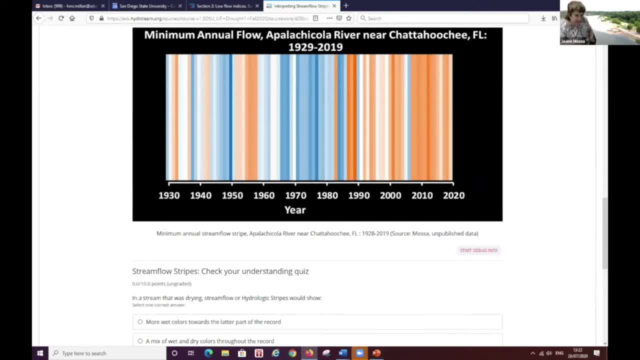 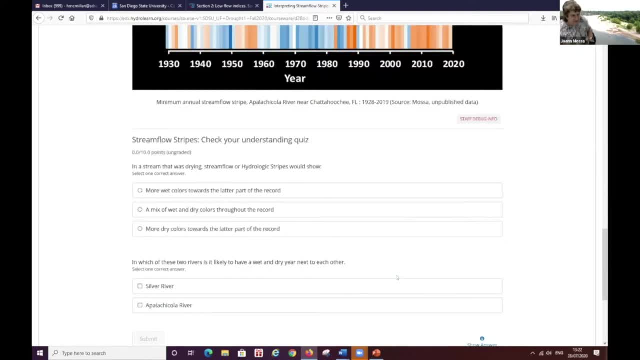 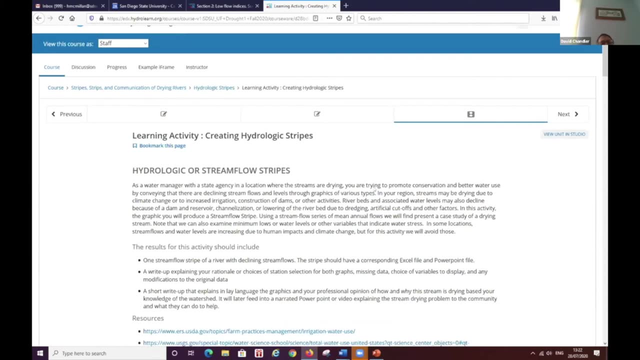 so why we have water wars with Apalachicola and Georgia and and Alabama, although I don't get too much into that in this at all. Um, let's go to, you know, the next one, I guess. And so here for the Learning Act. 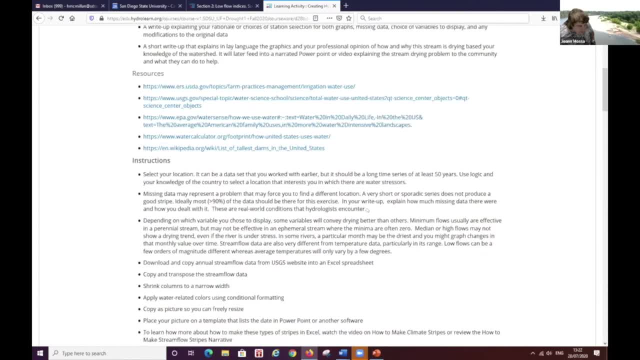 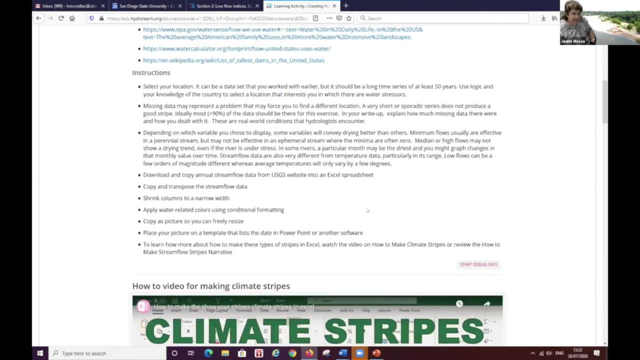 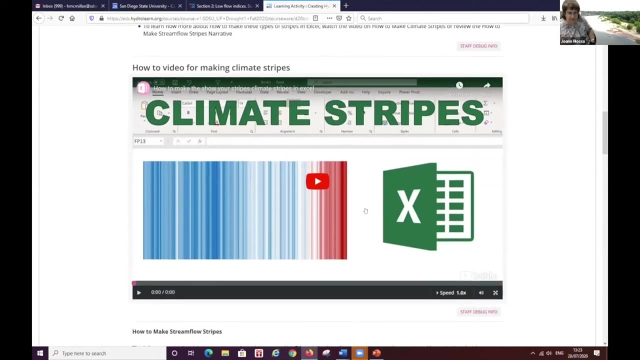 What's the question? Okay, so anyway. So through. we have instructions, we have ideas on how students can pick their own station by looking at where's the most irrigation, where's the most war. use all these kinds of federal links. 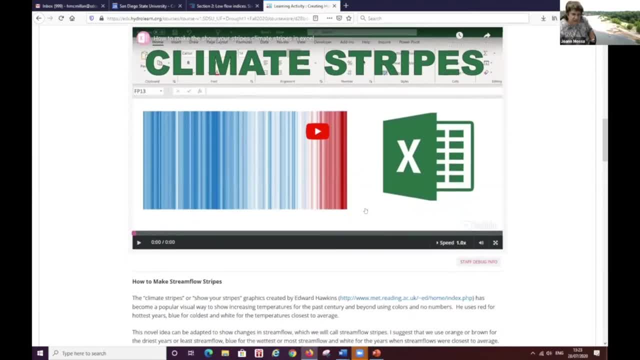 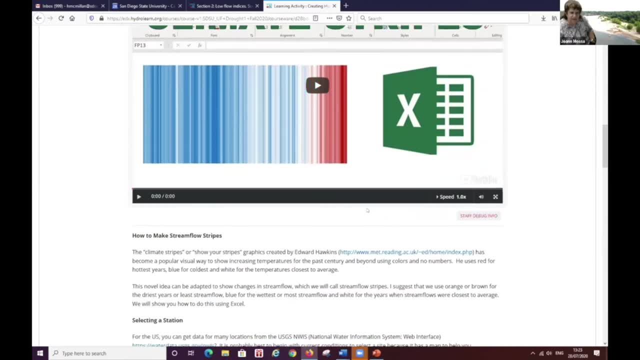 There's a video that a student made about how to do- or she a young woman, I don't know if she's a student- on how to make climate stripes in Excel, And that's one of the you know guides for the students. That was on YouTube. 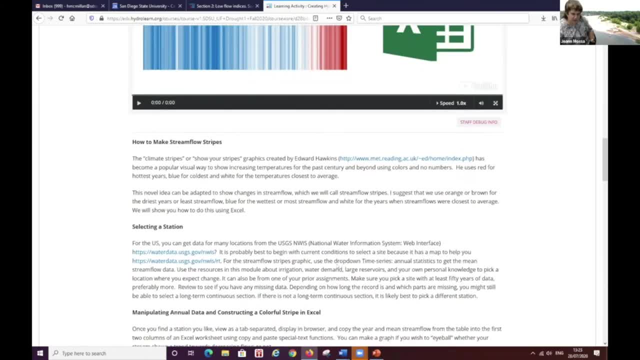 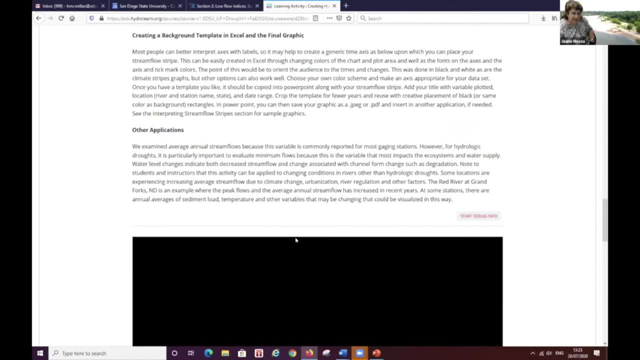 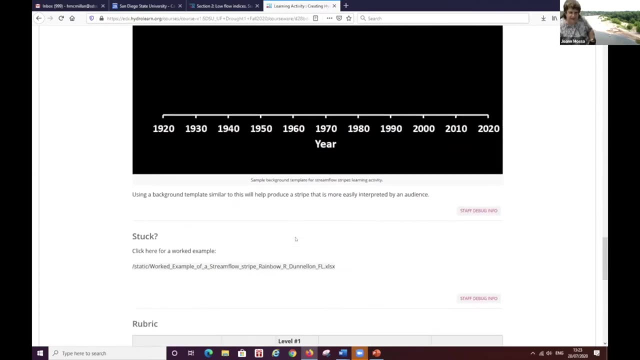 But I also have a specific how to make streamflow stripes And then go a little further. I've also encouraged them to make this a background template that looks like this, And then they plop their streamflow stripe on top of something like this So they can actually do time rather than just a series of stripes. 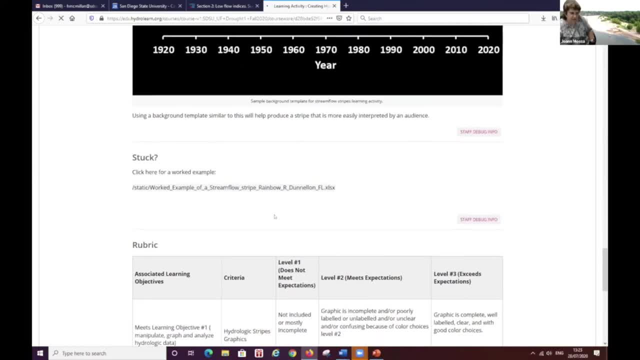 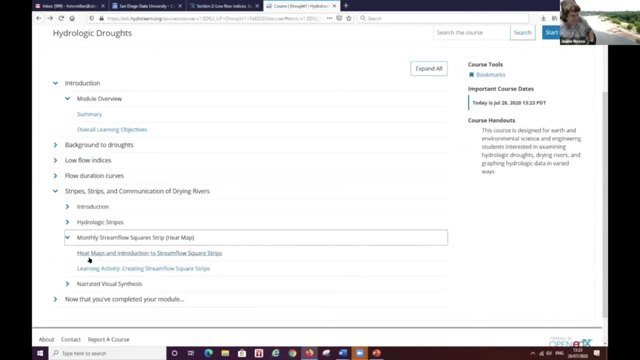 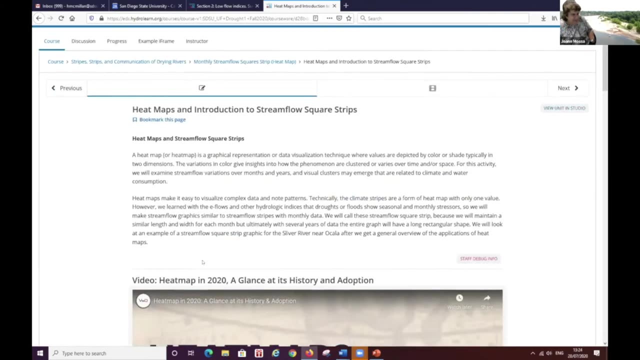 Um, so let's go to the next one, which is the heat map, or the strips. I call it stripes and strips. I call it stripes and strips Because they sound. it kind of goes together. And so the idea here is: yeah, let's go to the first one, So they learn a little bit more about the application of heat maps. 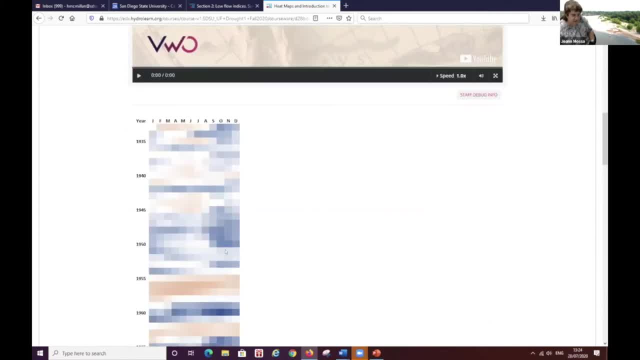 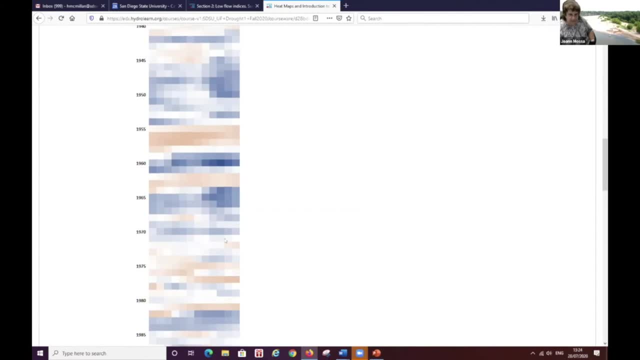 And, you know, one application, of course, is hydrology, And so I've created this, what other people would call a heat map. But again, the blue is the wet periods and the browns are the dry periods, And, as you're going through, 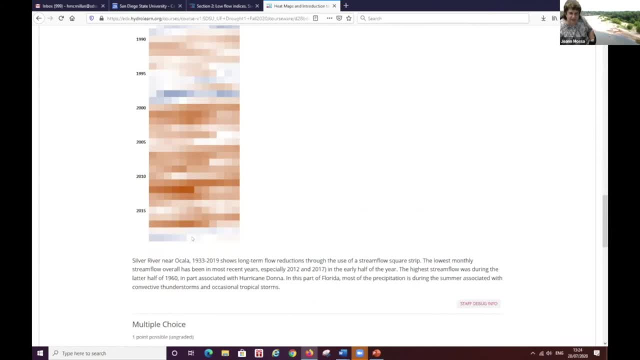 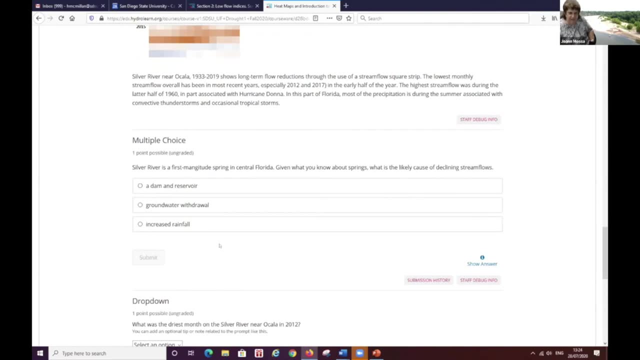 you know, 80 or so years of data. you can see this big chunk of dryness starting in 2000 due to, you know, taking more and more water of the aquifer. that's, you know, the river is getting less flow overall. 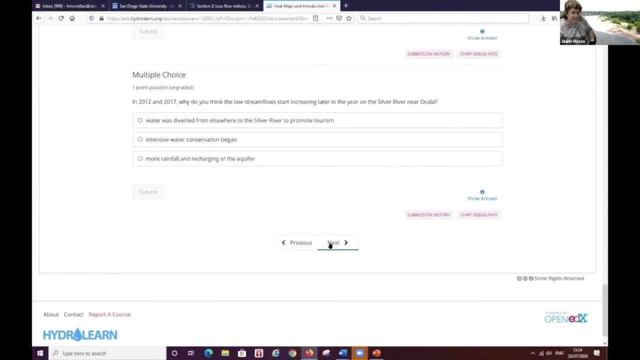 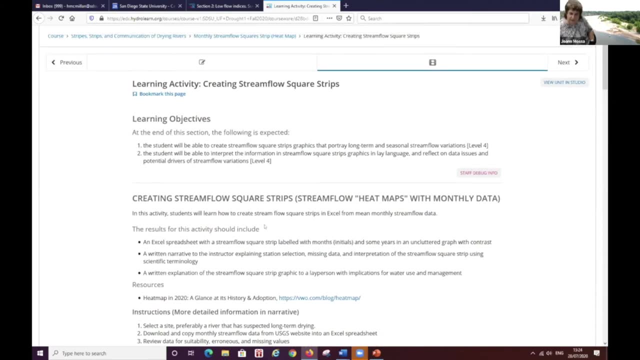 So just a few questions about interpreting this graph, and then the learning activity is actually creating this themselves, And this is a little bit more complicated. It can be done in Excel or Google。. So just a few questions about interpreting this graph, and then the learning activity is actually creating this themselves, And this is a little bit more complicated. It can be done in Excel or Google. 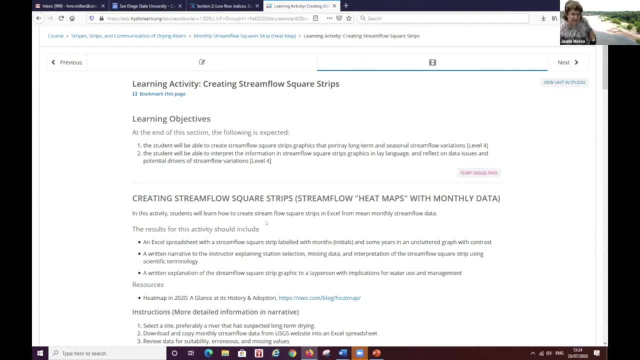 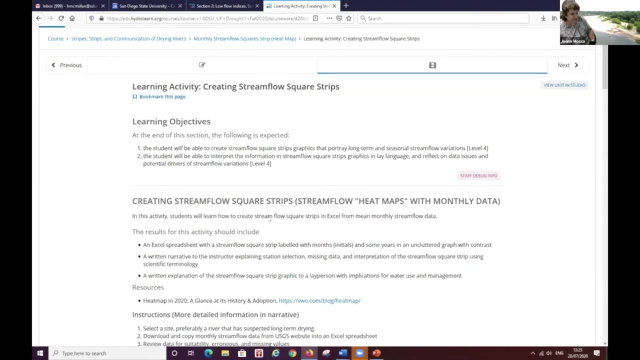 I give them the instructions in Excel and I give them again. they have a help at the bottom or, if they're stuck, they can see a sample sheet of how to do this. but this is a little bit more complicated because they have to use the VLOOKUP function and set up a couple of different grids to create this and so in. 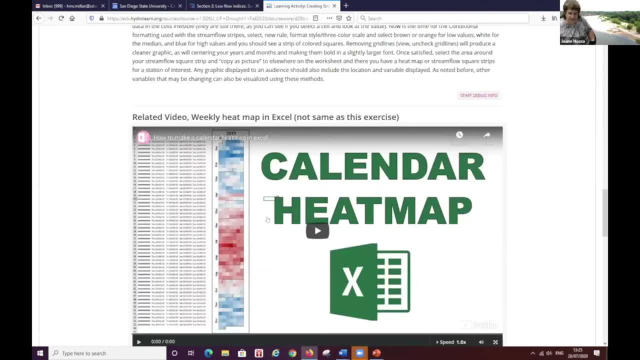 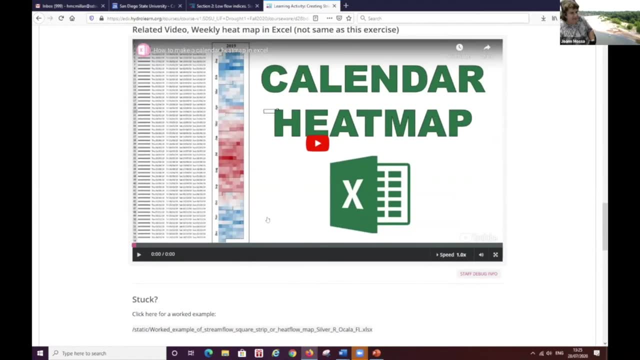 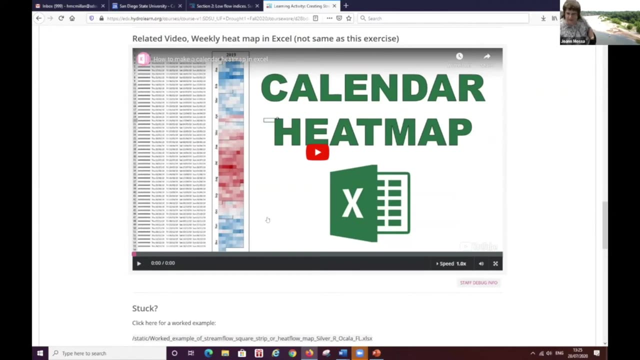 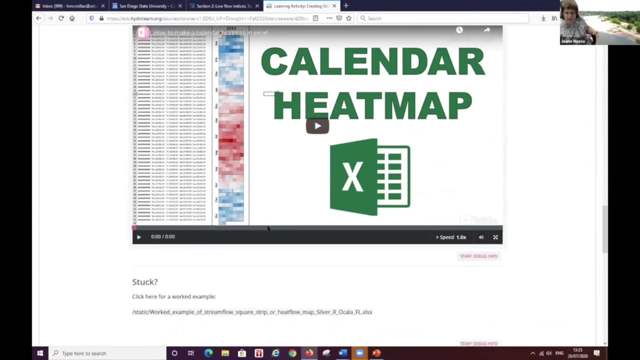 this case, they're much more likely to actually need resources. this video is, you know, somewhat related. it's kind of making a annual heat map from weekly data, and so it's not the identical project. but there's enough information in here that students also can see where the connection is. and again, I have a 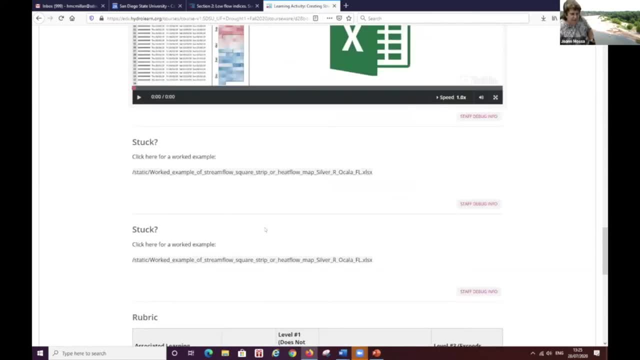 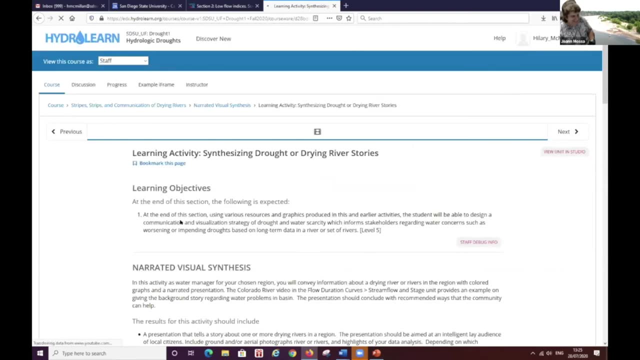 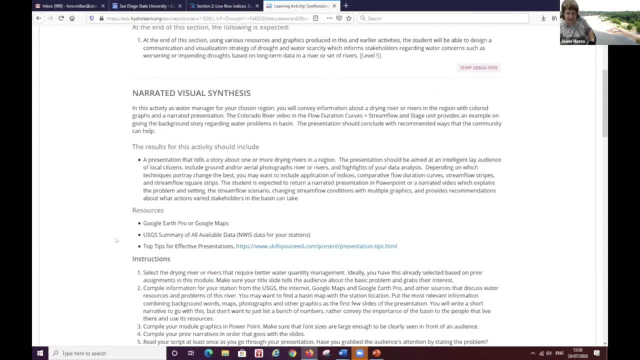 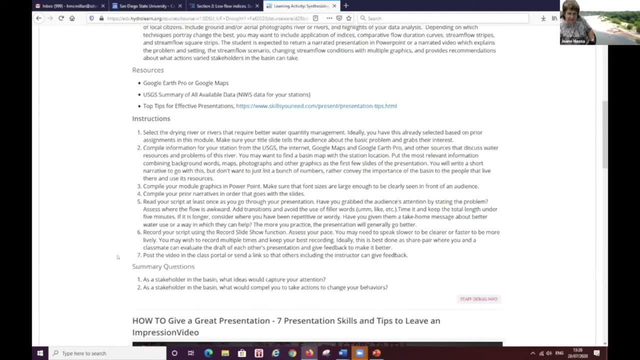 visual synthesis and they're the water manager trying to talk to stakeholders in this activity and they're choosing from graphics that they made or that they can create. you know of a particular stream system, that they have a case study and there is a video over here about how to give a strong presentation, like having a 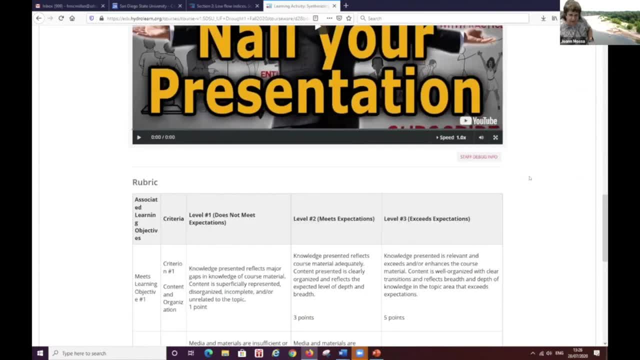 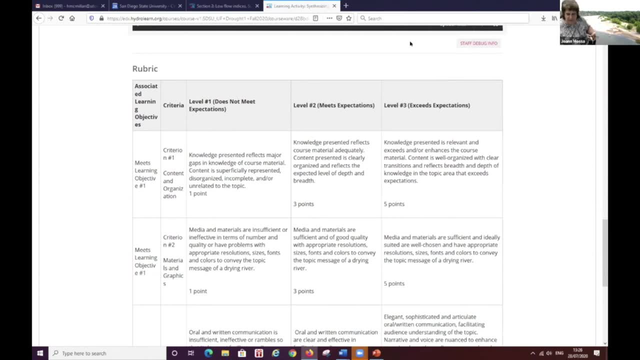 strong introduction to the water system. there is a video over here about how to give a strong introduction to the water system and you know having a take-home message and those types of things, but they actually have latitude about you know what materials they want to put together. that should. 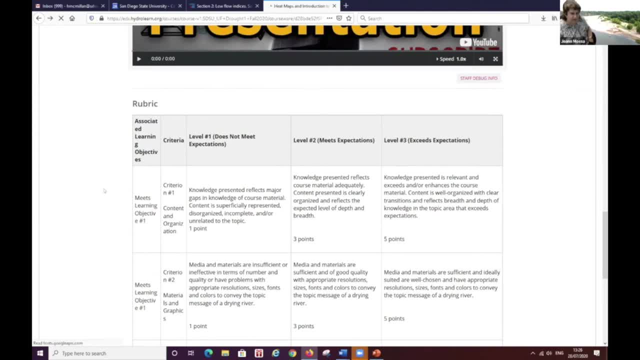 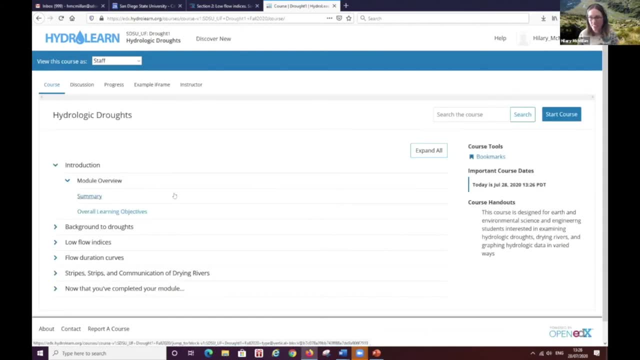 come from this material here and you know there's a rubric. so, Joanne, maybe we can give some time for questions, because we only have a few minutes left. I'm done, thank you. just like to hear what other folks think about it or if there's any. 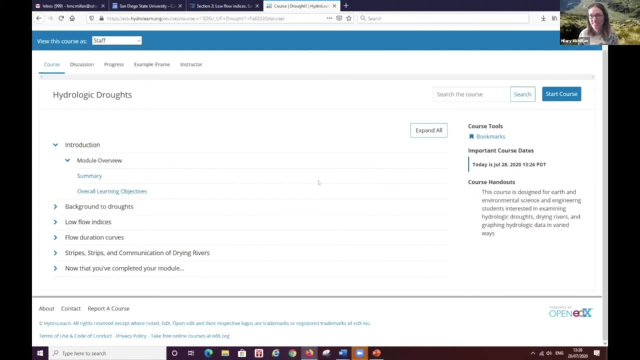 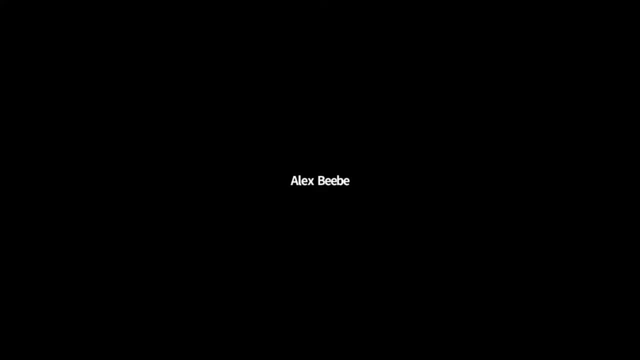 suggestions for how we can improve it. I'll stop my share because I can't see the chat. I've got a question. I really like this module. I could see myself using it my hydrology course with the Appalachicola example. is there any discussion on the? 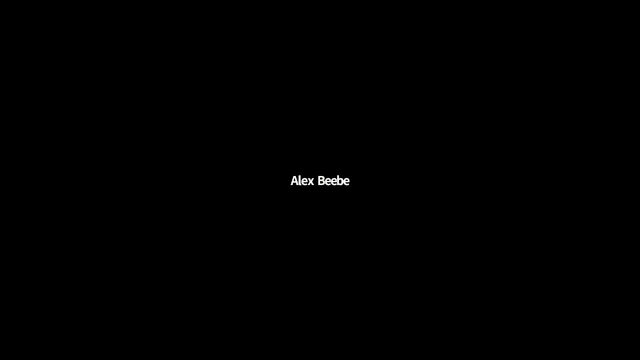 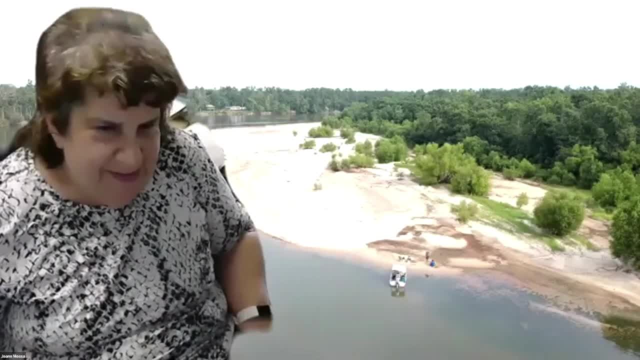 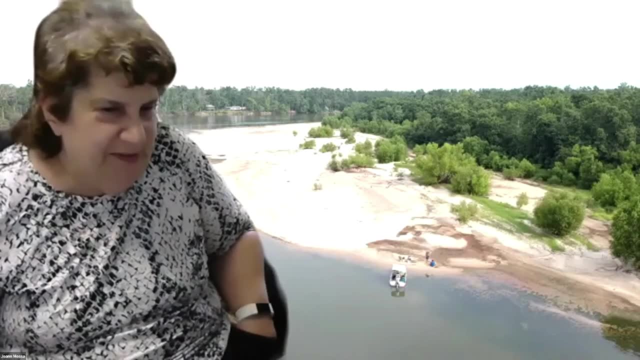 Yeah, somebody's posted a link there. Yeah, it is, And there's a lot of one. There's a lot of resources on that, So it's a question of how deep I want to get into it, Because it's interesting information, but it's not the. 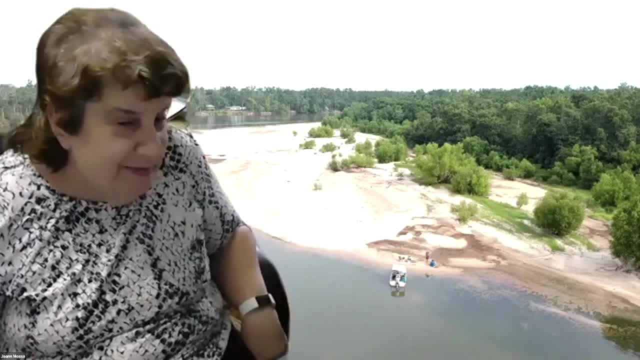 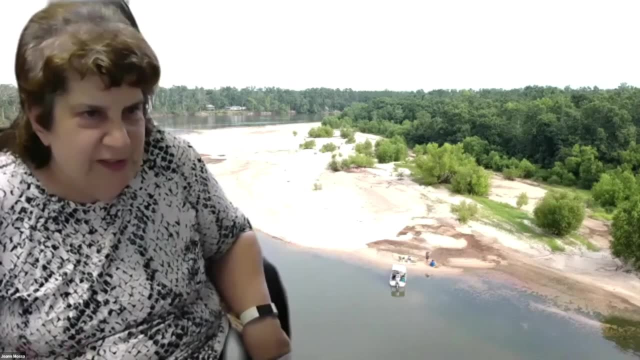 you know. so, yeah, I can enhance that, But I've actually published multiple papers on the Apalachicola in recent years. I have some EPA funding right now, And so I'm working on that issue and know a lot about it. 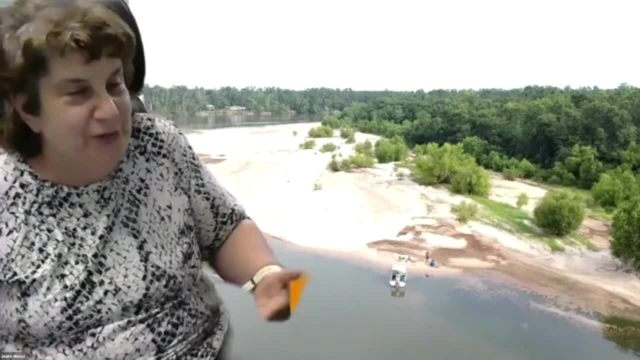 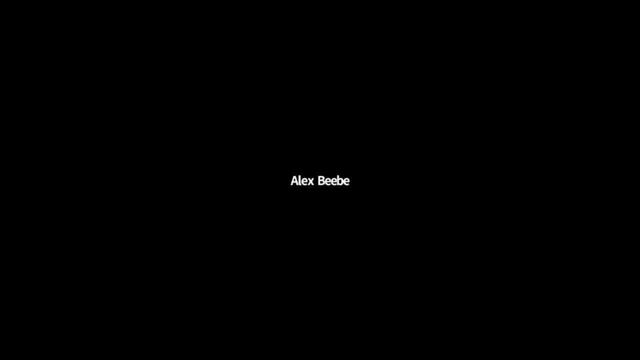 And I don't want to get too deep into it because I'm not sure how deep the students from California want to get into a Florida water problem. Yeah, I'm probably pretty biased because I'm in Alabama here, So I like seafood too. 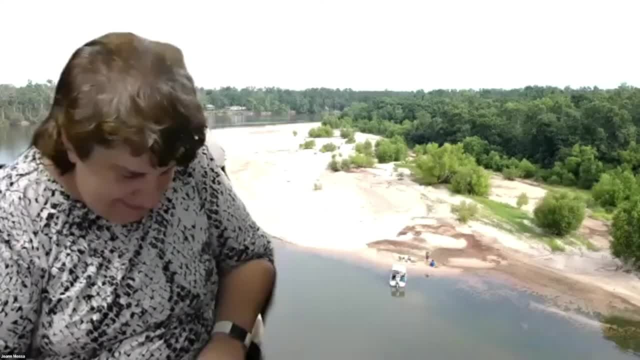 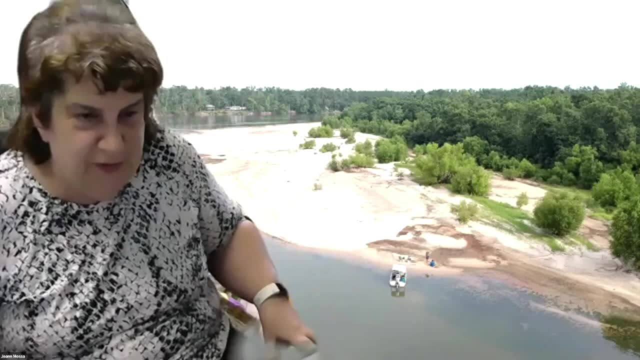 And I know a lot of the shellfish are affected by that too. Yeah, yeah, the oyster, the whole. you know there's a moratorium right now on actually harvesting oysters until 2025.. And you know there's a lot of right now. 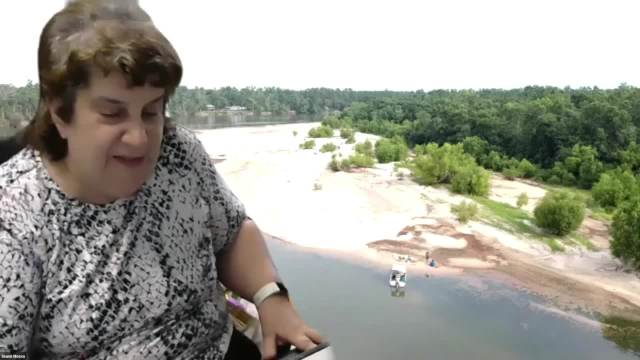 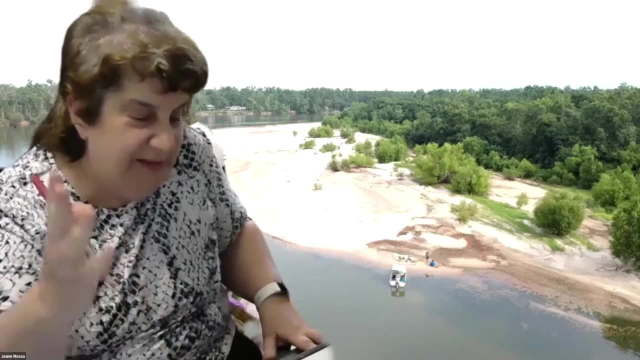 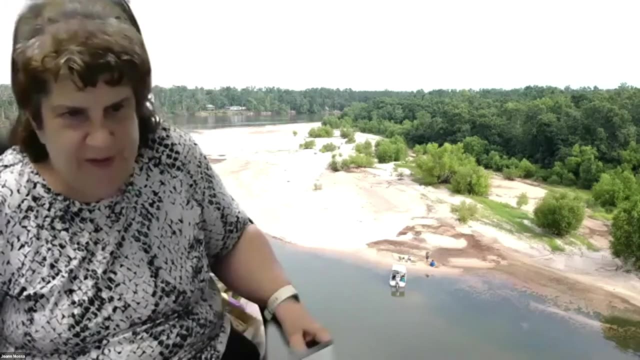 Georgia is, in a sense, winning the water war, Because unless we can prove economic damage of a serious degree, then they pretty much have total leeway, according to the last case about, you know, water consumption. So So I just moved from Atlanta. 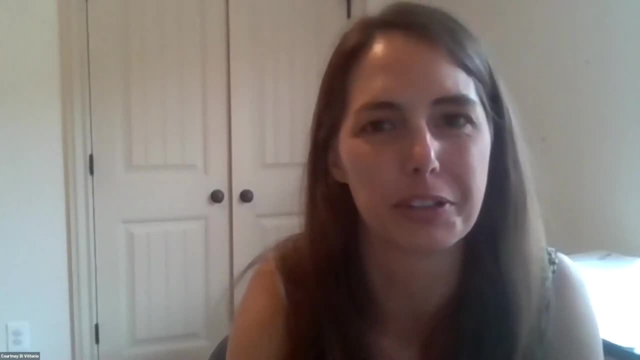 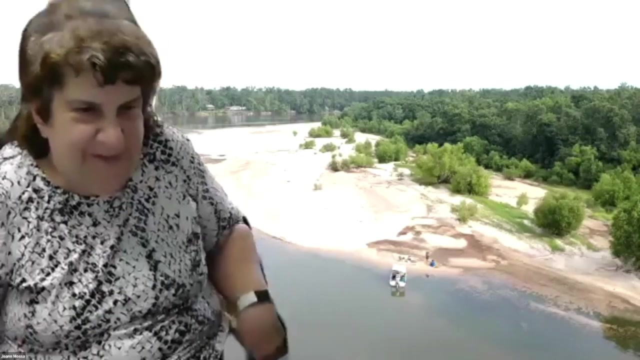 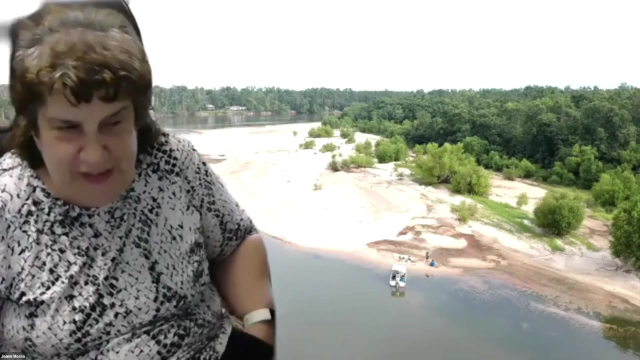 And my research group helped facilitate the stakeholder group meetings on the water wars. So we have Georgia, Florida and Alabama here. Yeah, we do, And yeah, you know different. I mean there are different issues in each area, you know. Georgia wants water for economic growth of Alabama too. Florida is mostly concerned with preserving the ecosystems. The upper Apalachicola is the highest area of biodiversity in the entire United States, So you know any water taken away can do serious damage to that. 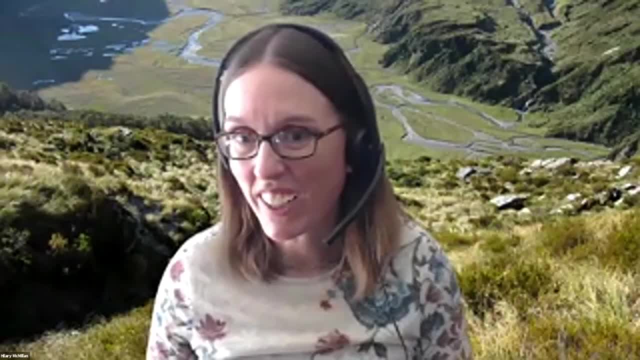 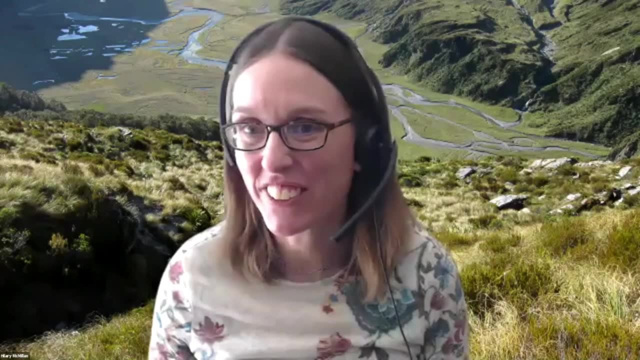 We have a question. Yeah, Hillary, Yeah, I'm answering some questions in the chat. So we had a question about the Q710 flows, which is one of the flows that's used for pollution control, basically kind of estimates: the minimum flow. 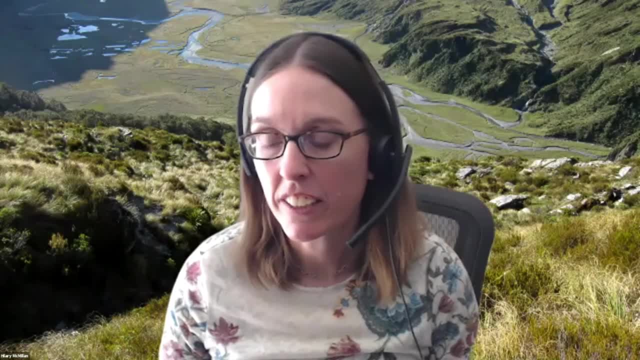 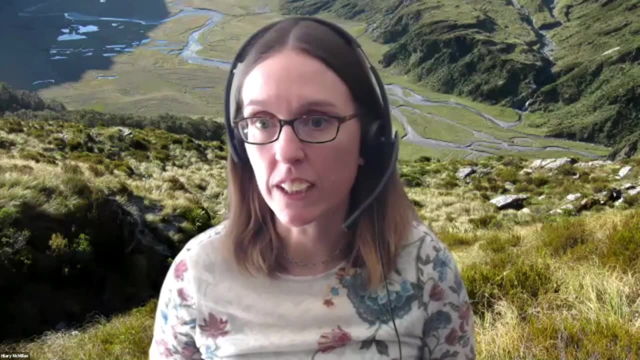 that you're likely to see in the river, which the students actually do calculate themselves using Google Sheets, because that's one that's quite possible for them to do themselves, Although I would have to say that this also causes a few problems, because many of the streams 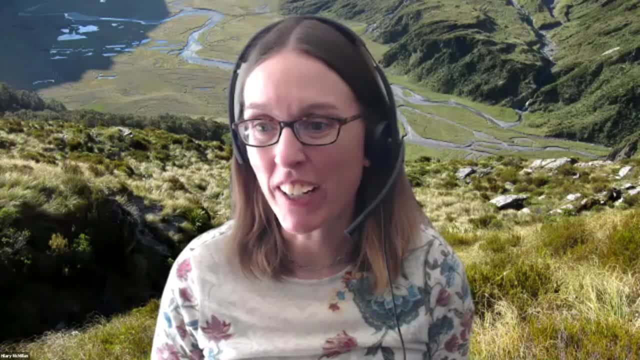 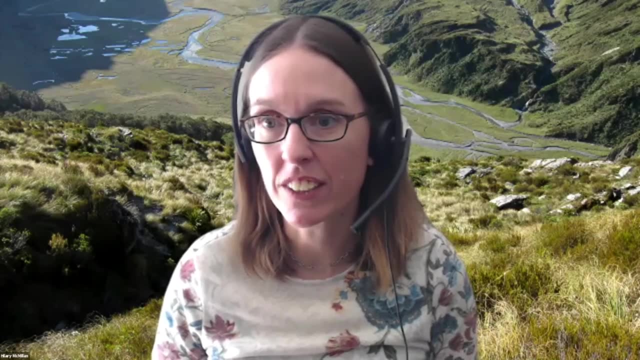 that they may choose. they might dry up totally at some point, in which case you just get a zero value there or they have missing data. There's sort of some description which messes up when you're trying to calculate absolute minimums. 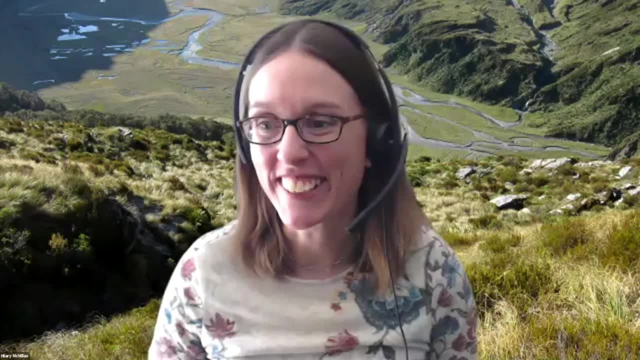 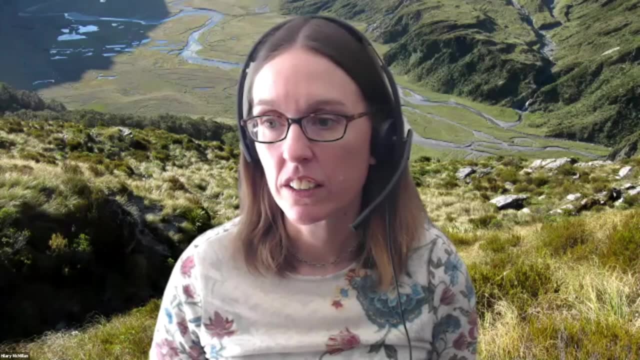 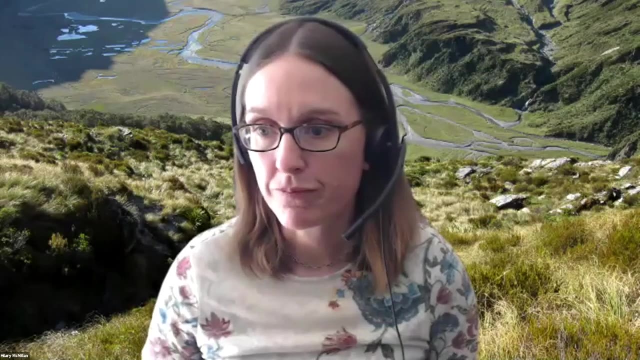 So it does cause a few problems, But we encourage the students to check out their data carefully before calculating these indices, And I think we'll also need to talk to them about the suitability of different indices for different places and for solving different problems, Right. 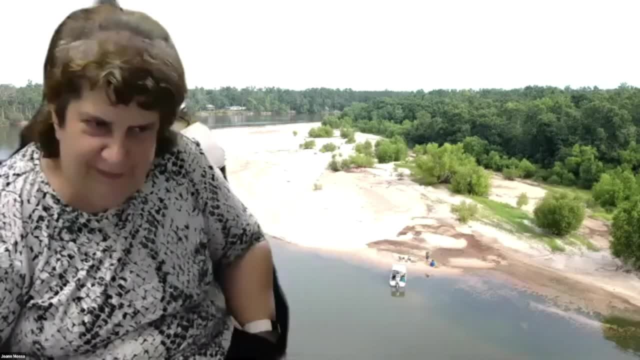 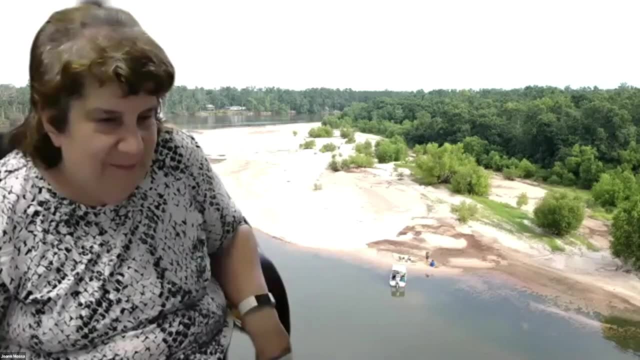 And I have them also look for missing data and not go ahead at some point if they have too much of it. So I think that's a good way to start. So I'm going to stop here And somebody asked about: oh, here we go. 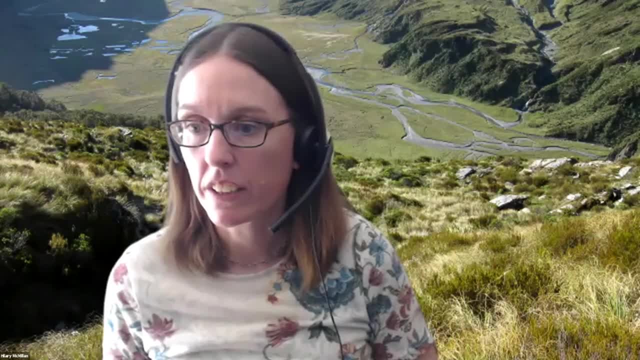 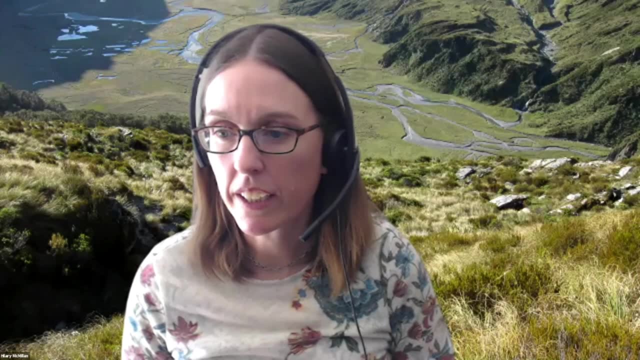 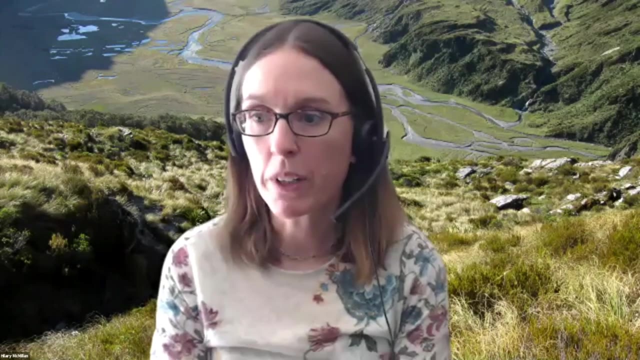 how much probability or stats background. There's not very much that is involved here, I guess. Just trying to think what they need to know, I had to introduce them to return periods for things like the Q7-10.. So they need to know how to estimate those. 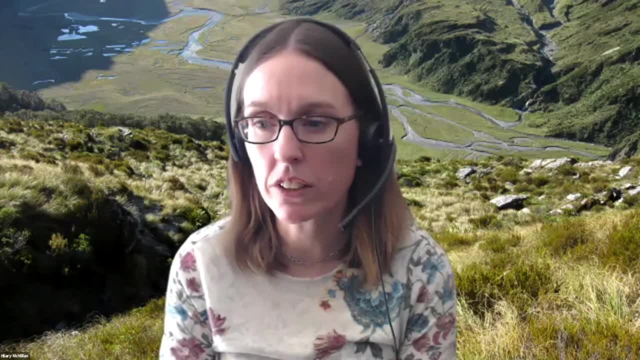 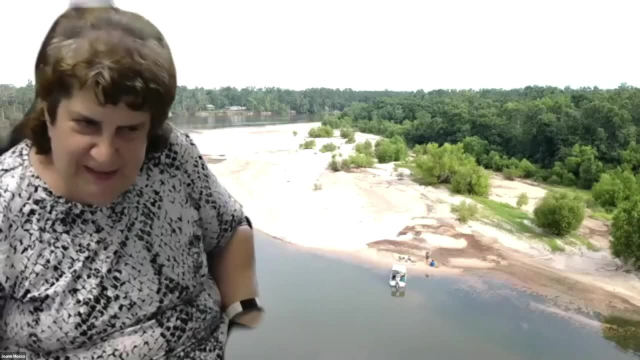 So I provided a little bit of background. Maybe Joanne you can speak to. did you provide some background on what is a CDF before they get into flow duration curves? Very basic details about the and maybe that could be an area. 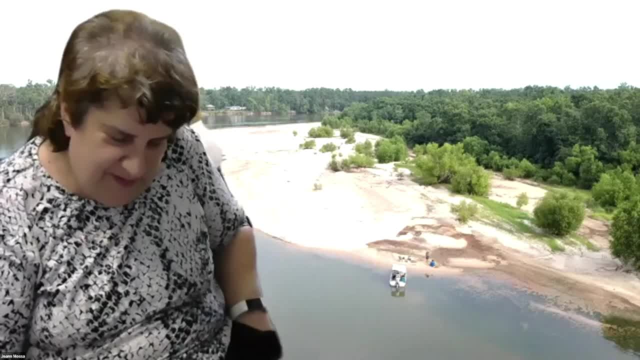 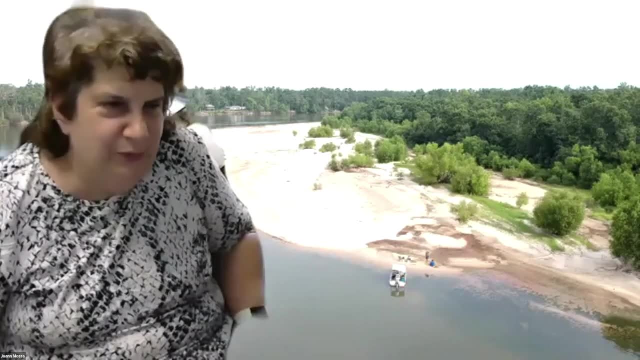 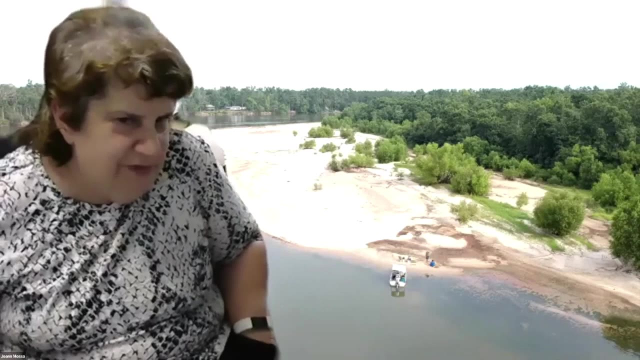 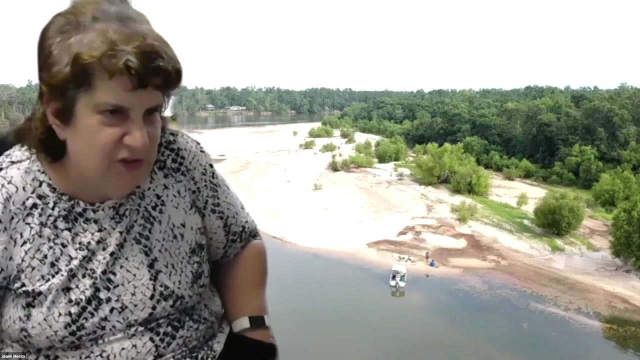 that I could actually enhance in our revision. So this is the feedback process, But I did describe what the purpose of it was and what it was essentially. But we can go And if someone thinks I should really go, take a deeper dive or explain more, that's something we can do at this revision stage.